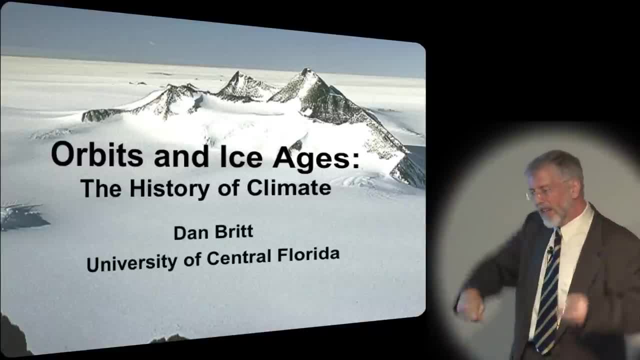 on all the walls and down the center with glass tubing and beakers and Bunsen burners and stuff bubbling over and big machines with lots of flashing lights. It was a science lab for central casting And what they did was, amongst other things: 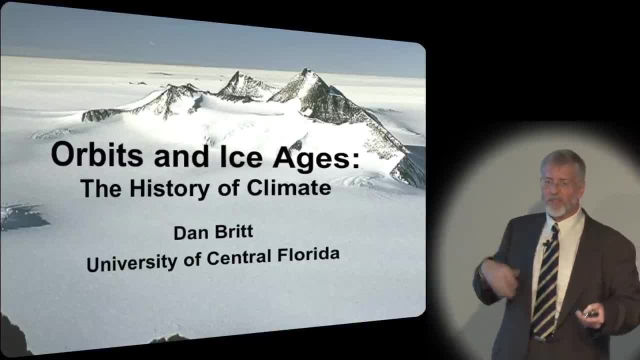 they measured the isotopic ratios of ice cores. and that's what I did for three years, And for three hours a day, three days a week, I would stand in a freezer and cut up ice cores and then go measure them in a mass spectrometer, you know. 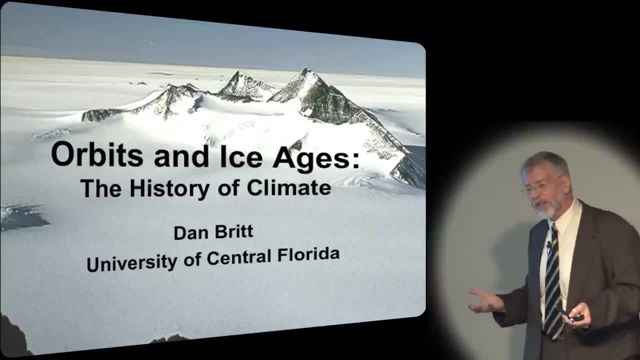 Here I was, you know, middle-aged undergraduate, no experience in science, and I said I want a job running a mass spectrometer And for some reason they let me do it, And so a lot of the data I'm going to show you today. 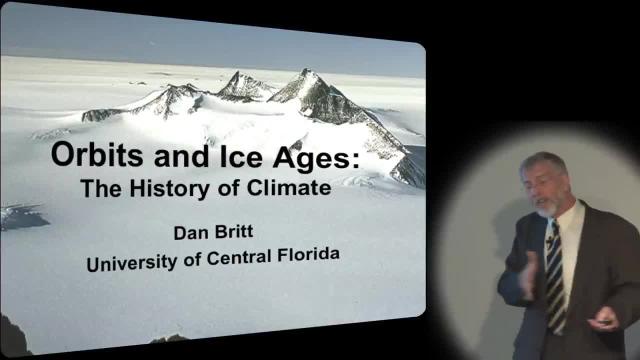 I actually took, Which is kind of cool because I was at I attend scientific meetings. later and years later I was sitting in a meeting and some of the data I took flashed up on the screen And in the question and answer period. 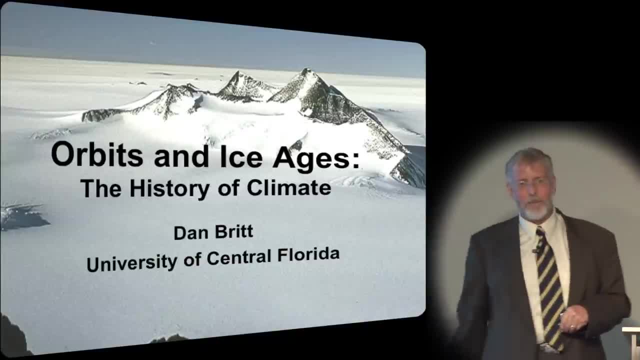 somebody got up and said: I don't believe that data. It looked like they made a bunch of mistakes, And so I got up right behind them and I said: I took that data And we noticed the trends that you noticed, because we're not idiots. 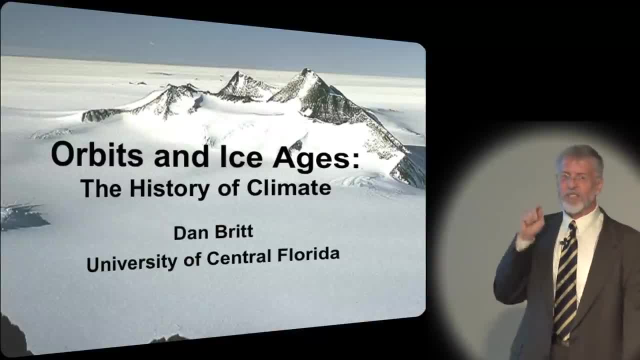 But we checked it over three times and that's reality. Just because you can't figure out reality, that's not reality's problem, That's your problem, And I'll be happy to discuss this with you outside. I'm kind of I believe in kind of a muscular science. 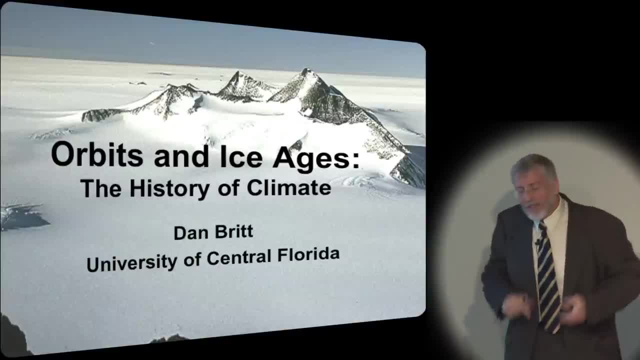 I've always wanted to do that, Anyway, so I'm going to show you a bunch of stuff. The problem is with climate. there's a lot of things going on. This is not soundbite science, So I'm going to tell you a lot of complicated stuff. 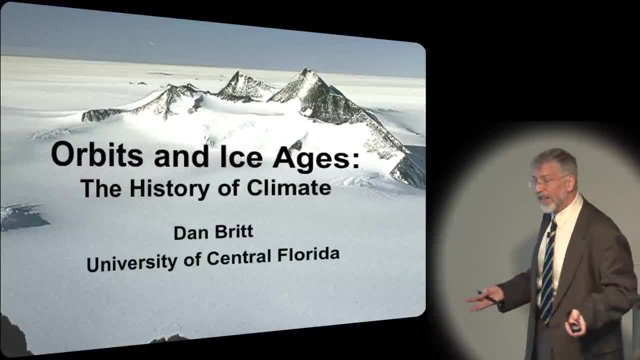 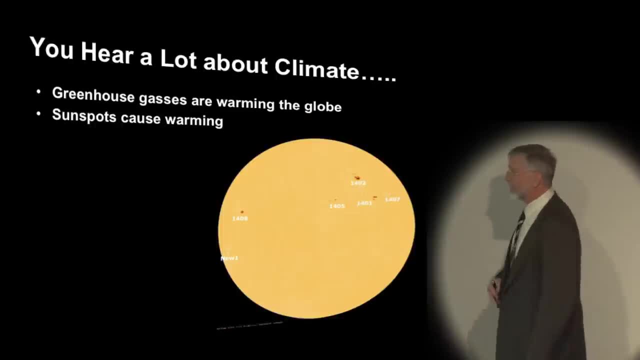 I'll try to be entertaining. Some of it will be boring. I apologize in advance, But with climate you hear a lot of stuff. You see, greenhouse gases are warming the globe. Sunspots actually cause the warming. These are actually the sunspots from Tuesday. 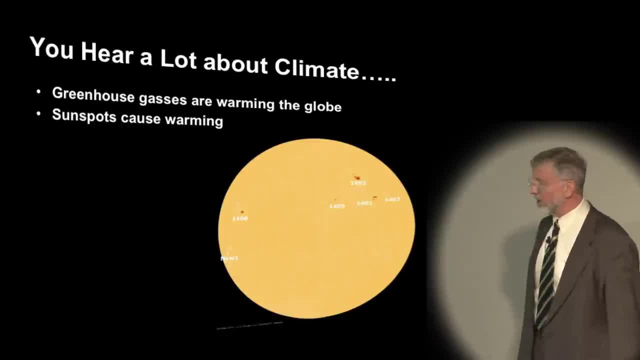 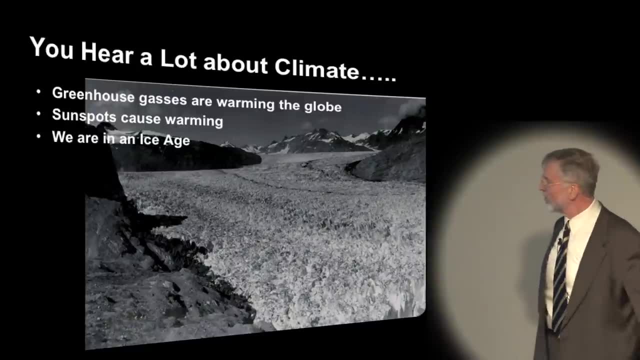 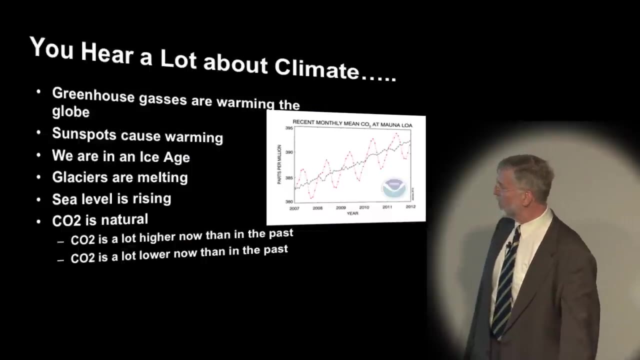 I doubt you could. there's a NOAA site that you can go to and get the latest sunspot data. That's the latest sunspot data: That we're in ice age, That the glaciers are melting, Sea level is rising, CO2 is natural. 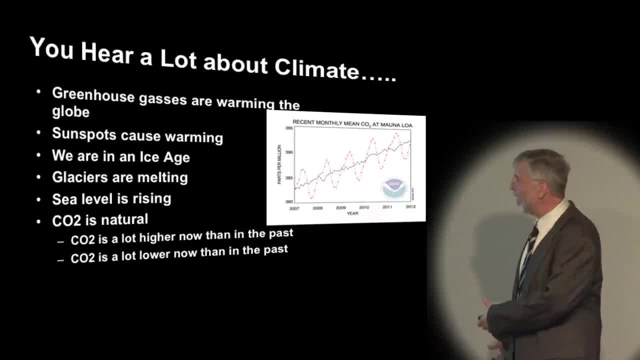 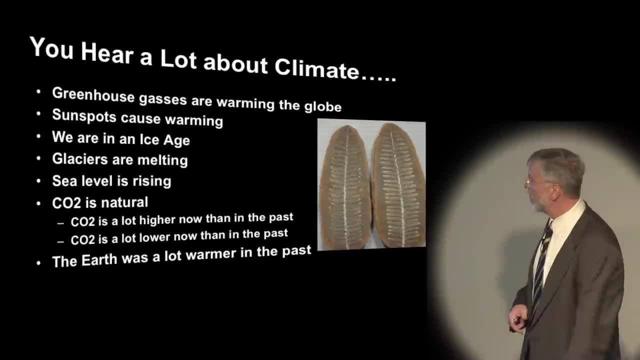 CO2 was a lot higher in the past. CO2 was a lot lower in the past, That the Earth is a lot warmer in the past. The Earth was a lot colder in the past, And the problem is that everything here is true. 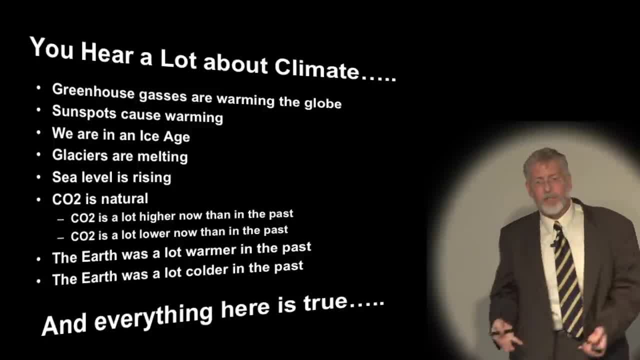 Sound confusing? Well, no, it's not. Actually, it's quite reasonable. The thing is, we actually know quite a bit about past climates. This is what I did in this laboratory. Now I can go into excruciating, mind-numbing detail. 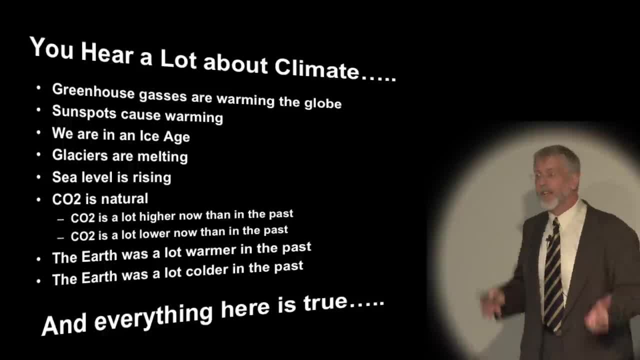 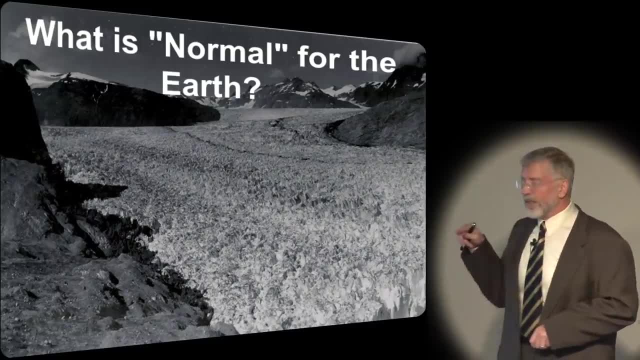 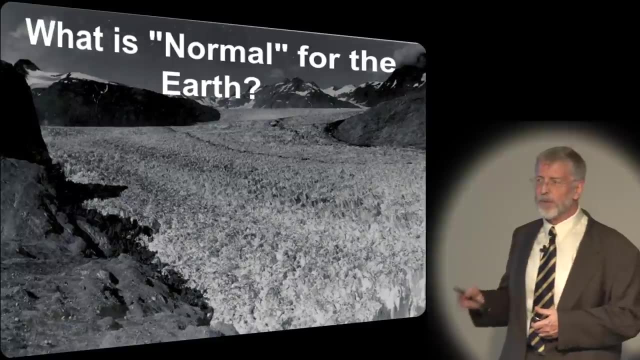 as to how we know it and the physics behind it. I will spare you that. If you insist, I will tell you Okay, But what this does is it tells us we know the Earth's climate history pretty damn well for the last half billion years. 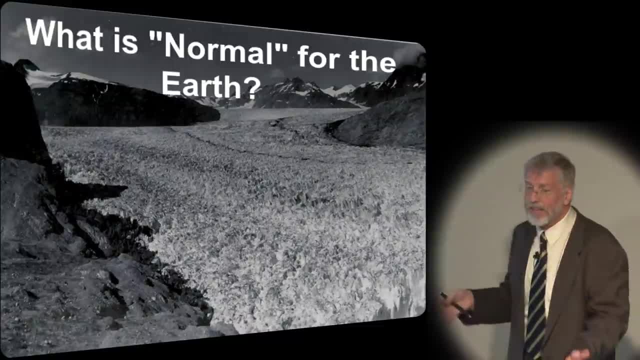 After that it gets a little tricky, But for the last half billion years, I mean, it's a lot And that's not bad. And so we can actually look at what's normal for Earth. And the question is: what is normal for Earth? 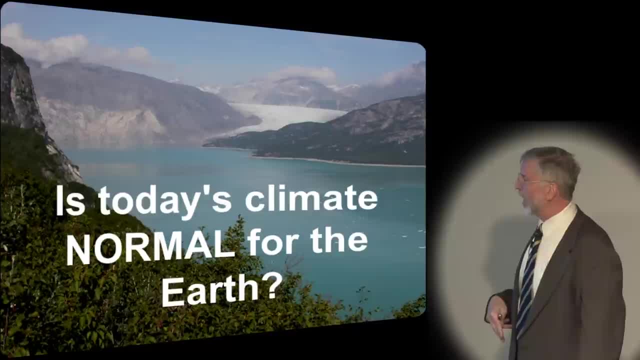 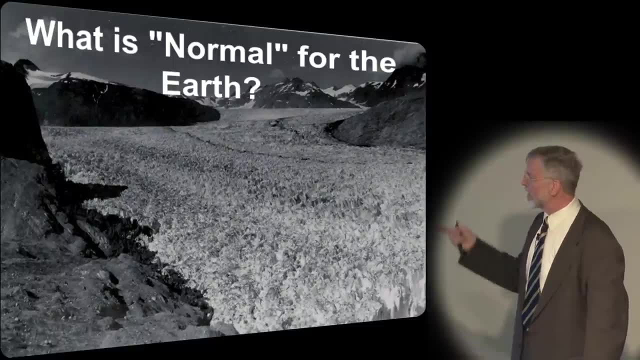 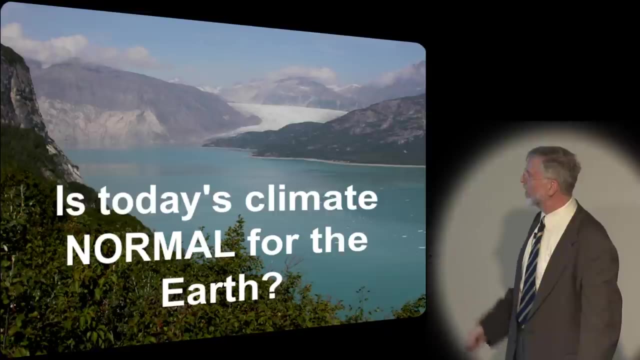 Is today's climate normal for Earth? Now, actually, I like this picture because this is the same location. There's about 60 years difference. here You can see the bathtub ring left by the glacier. right there, See, right there, See, right there. 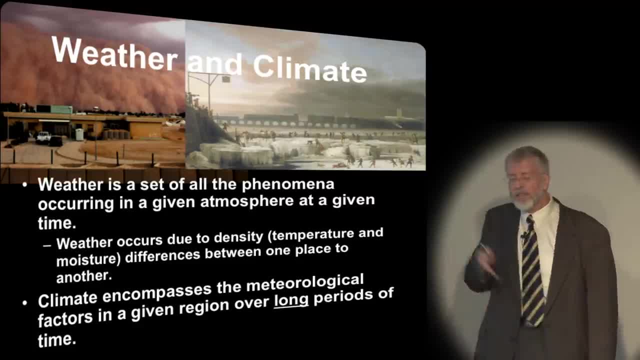 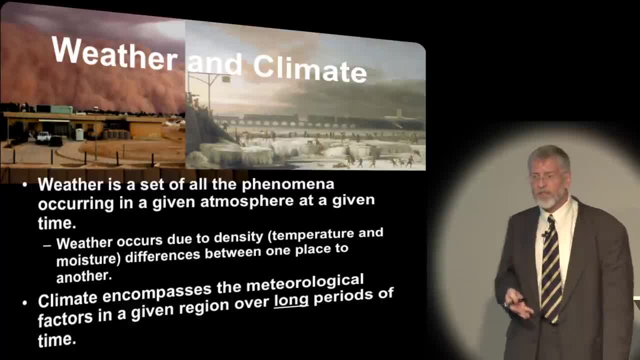 That's way beyond my abilities, because that is hard. There's a reason why people don't forecast hurricane tracks more than five days in advance: Because that's really, really hard. I don't do weather, I do climate, And when I talk about climate, 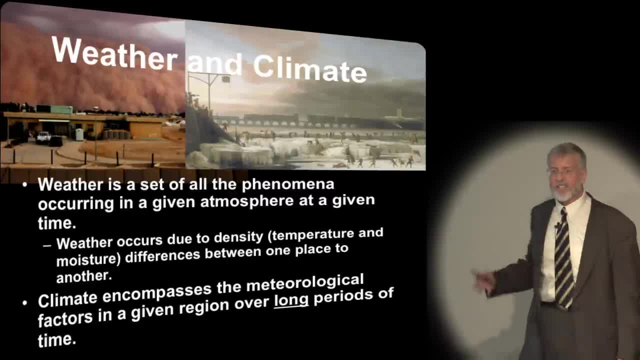 I talk about land, I talk about long-term climate, Climate in geologic terms. And in geologic terms you can actually find out the effects, because this climate experiment has been done over and over again in Earth history And all you have to do is go back and read the rocks. 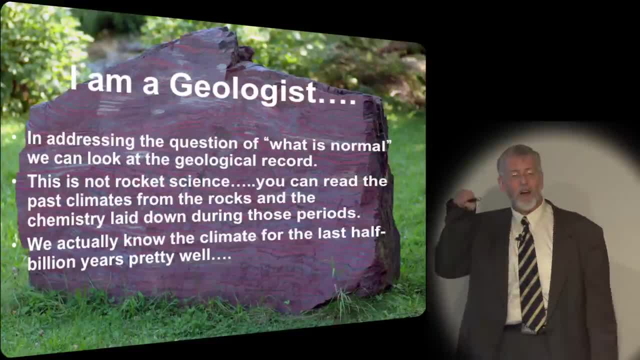 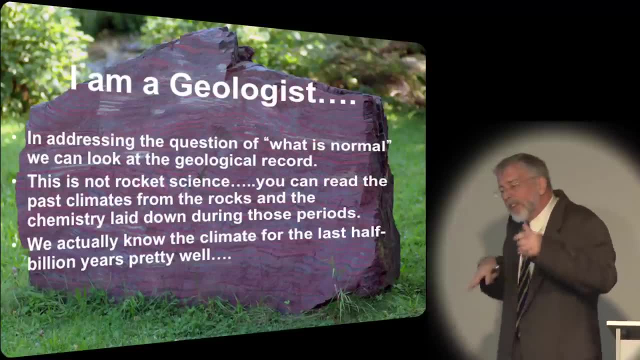 And that's what I do, Addressing the question: what is normal? All you need to do is go back and look at the geologic record And how things change with changes in the various climate parameters. all you have to do is go back. 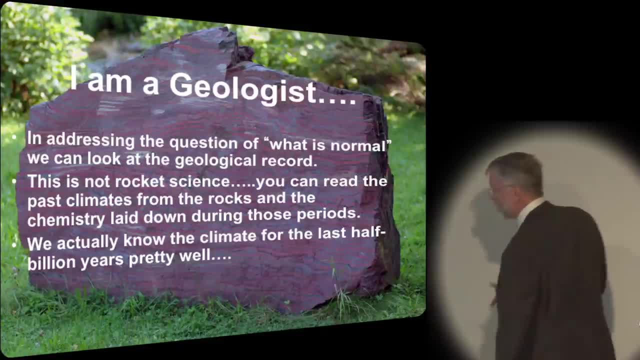 and you can read the past climates from the rocks and the chemistry laid down in those periods. And the nice thing is that people that are a lot smarter than I have have puzzled this out And a lot you know- have a lot higher tolerance for boredom. 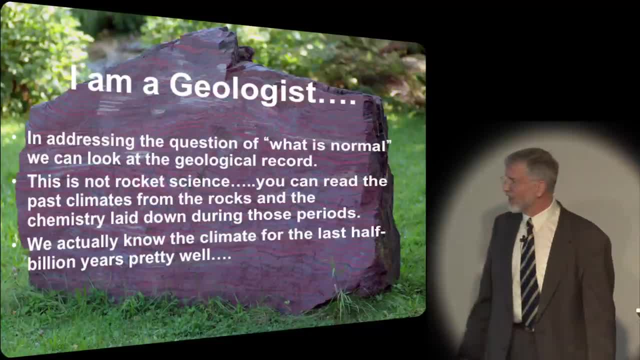 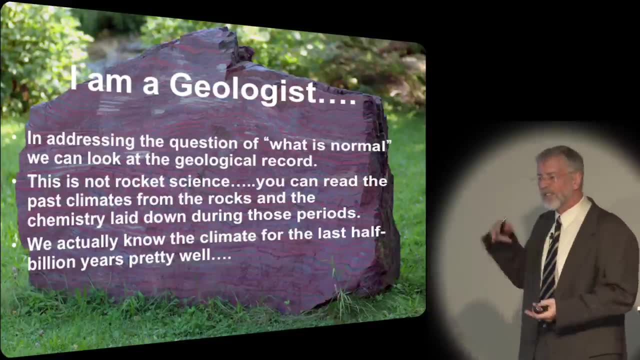 And so they've done this over the last half billion years, And we know this pretty well About as well. you know, remember, science is tentative Science. we're always groping for answers and testing these answers. So you know, we know. so there are various grades. 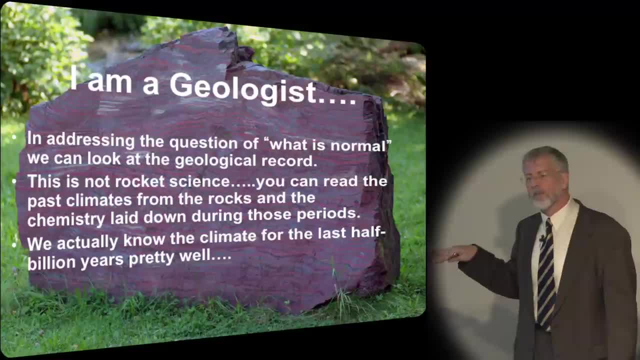 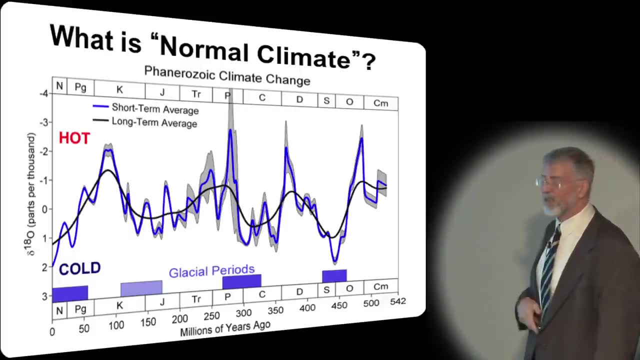 of how well you know things. This is a pretty high grade. We know this pretty well, And so what's normal for climate? This is phanerozoic. Phanerozoic is what you live in today. That's the period when you have, like, complex critters. 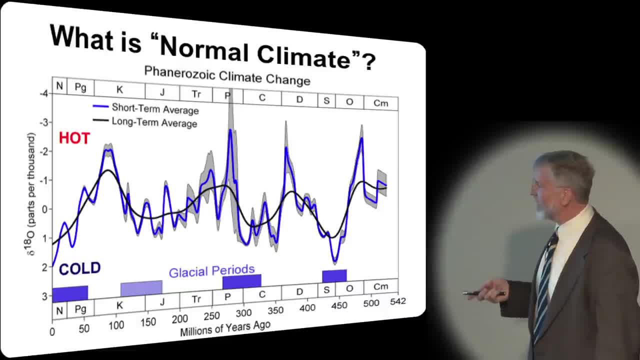 We are here at zero in the neogene. We're gonna go back a half billion years And the first thing you see is that it is about as cold right now as it has ever been in the last half billion years. We are actually in an extraordinarily cold period. 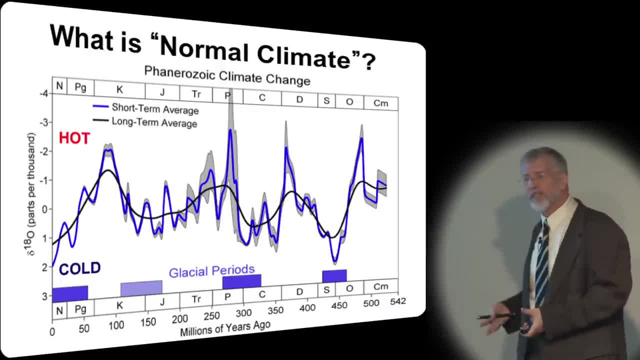 We are in an ice age today. We're in a relatively warm period of an extremely cold period. You know, I didn't say this was going to be easy. This is, this is, you know, reality is just. I'm not gonna sugarcoat reality. 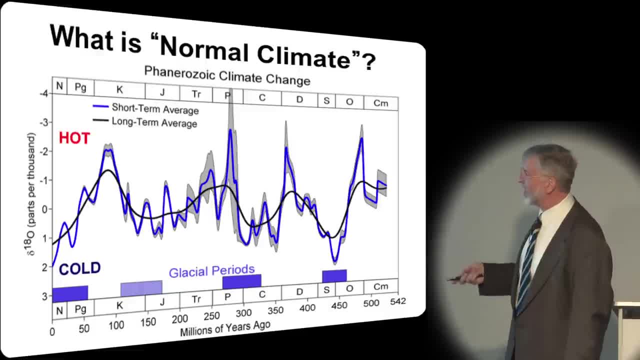 This is reality, And so we are very cold. Back during the Cretaceous- the K means Cretaceous- scientists don't spell well- It was extremely hot, But average for Earth is a lot hotter than it is today. But what you should take away from this slide: 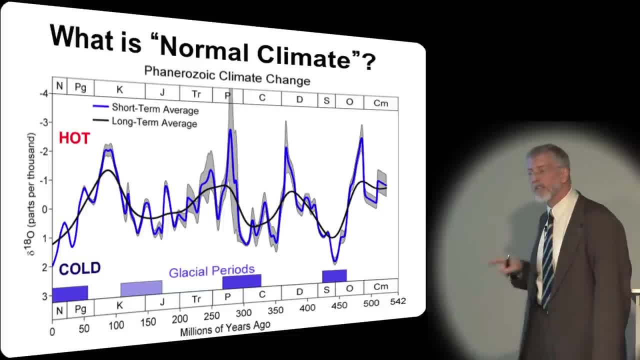 is that there's nothing normal about climate. Climate varies a lot, And it varies a lot for very good reasons, which we can figure out and which we will figure out tonight. But what were things like in the Cretaceous? Cretaceous with a C. 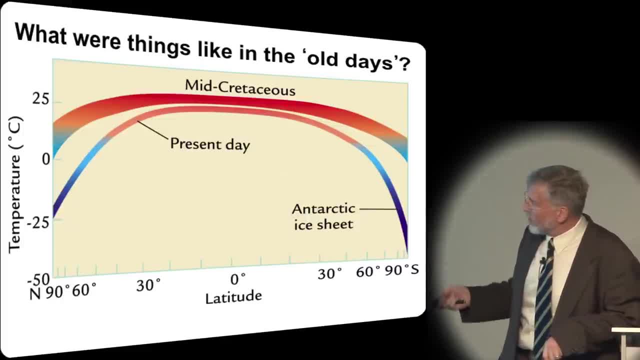 Back in the mid-Cretaceous. this is the temperature profile by latitude We are at. we are about right there, about 30 degrees. So actually the climate for the latitude of Pensacola was not all that much different in the Cretaceous than it is right now. 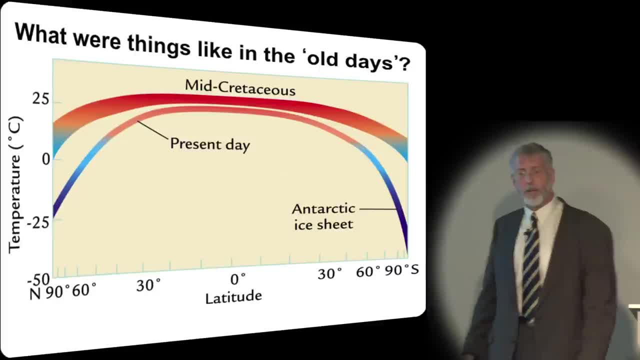 It's pretty warm, Not unbearably warm, because, you know, with a little bit of air conditioning it's very pleasant to live in Pensacola. But it's much different than the present day, And the difference is not in the low latitudes. 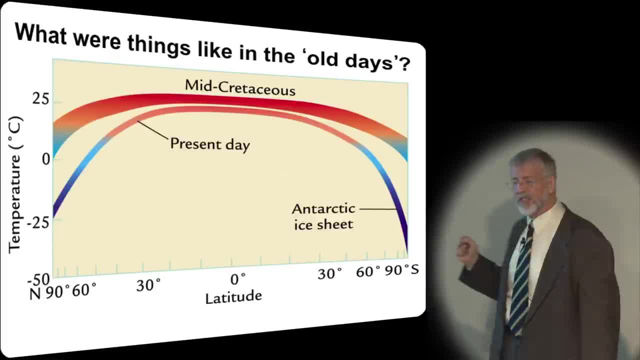 It's in the high latitudes, Because in the Cretaceous, nowhere on Earth, even at the poles, was it on average below 30. Below freezing. if you can imagine that In the Cretaceous you had a temperature profile. 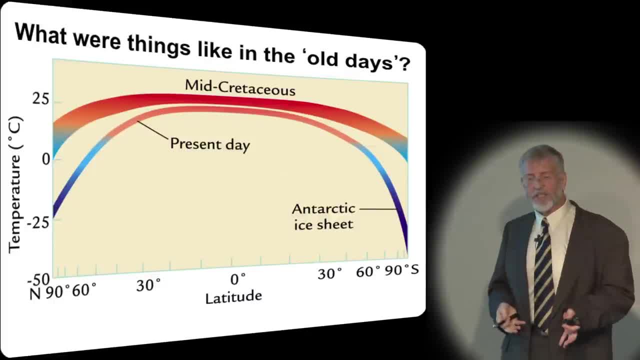 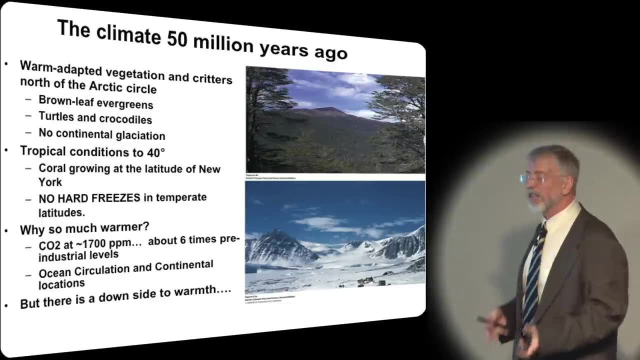 that essentially made what you consider temperate climates, going all the way to the Arctic Circle. So in the Cretaceous you had warm adaptive vegetation and warm adaptive critters at the Arctic Circle You can go to the Arctic Circle today in Canada and find. 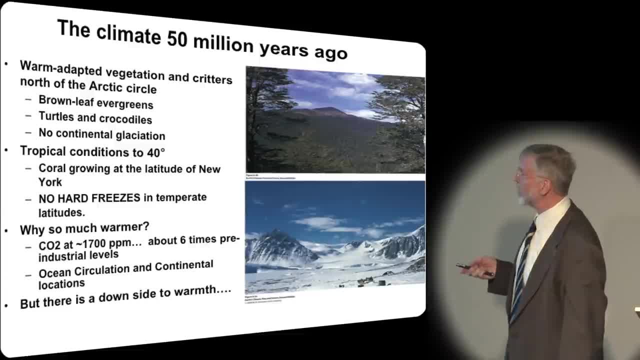 breadfruit tree fossils, fossils of turtles and crocodiles, And there was no continental glaciation anywhere, Not even the poles, not in Antarctica You had tropical conditions to 40 degrees north-south latitude, So that's the same latitude as New York. Can you imagine the climate of Key West in New York City? Coral reefs growing off of Long Island. No hard freezes in Ohio. Can you imagine Ohio without hard freezes? People would want to live there All year round. I can say this about Ohio because I've lived there. 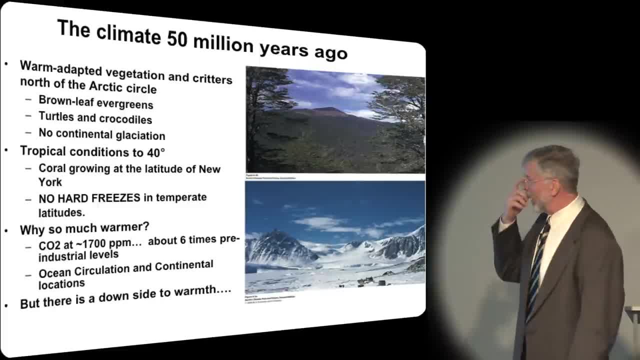 I don't want to insult Ohio. Ohio is a wonderful place to live, But they have hard winters. This is you would have essentially the climate that you enjoy in Pensacola in Ohio. Why so much warmer? Well, back then, CO2 was about 1,700 parts per million. 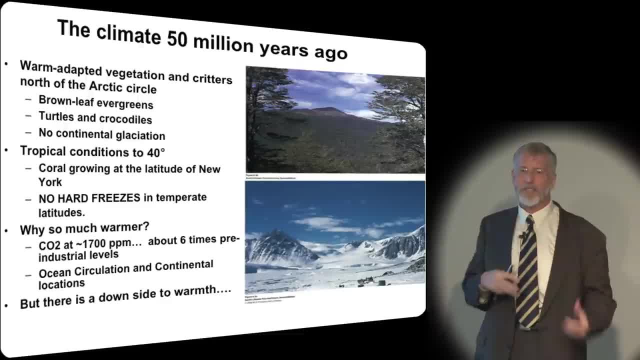 Now this doesn't mean a thing to you right now. You will know these numbers at the end of this lecture in great detail, because I will keep repeating them to you. That's six times the pre-industrial levels of CO2 that we enjoy in the recent period. 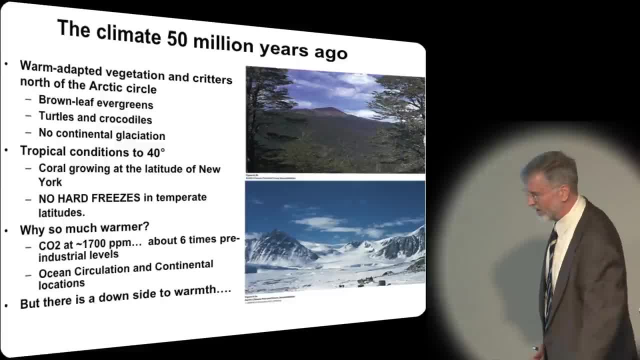 And remember, when I talk about recent, I'm talking as a geologist, So this is over geologic time. I consider the recent period, the last 10,000 years. This is just my quirk, So when I talk about the old days, you know. 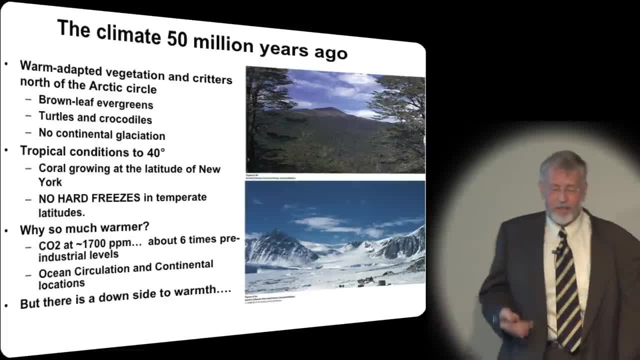 the old days are. you know something like that. I'm talking about a year, you know, 70 million years ago, You know? the other quirk is that I just don't, I don't, I'm not interested in things. scientifically. I just don't have interest in things that haven't been dead for half a billion years or so, But now that's another story Anyway. so why so much lower, Much higher CO2, a much different ocean circulation in continental locations? 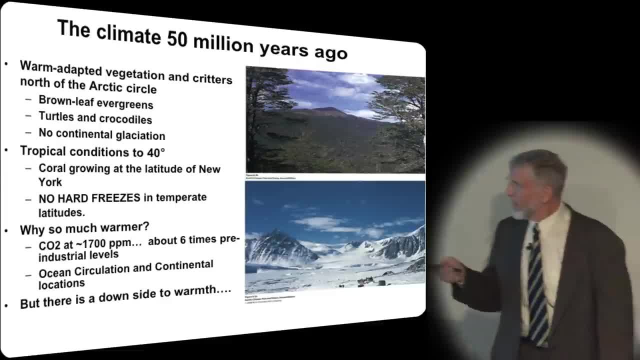 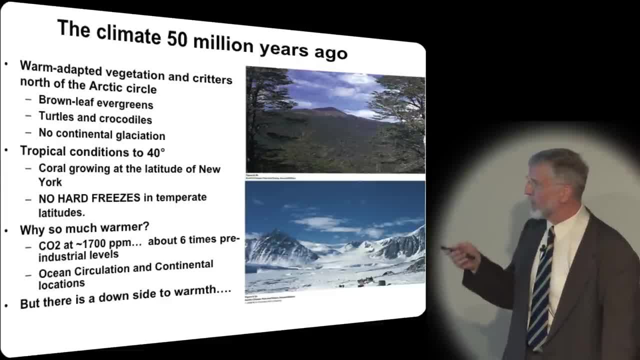 this was you know, this was you know, this was you know, this would be in the Cretaceous. versus now this would be the same location, This kind of vegetation which today it looks like that. The downside, of course, is that no continental glaciation. 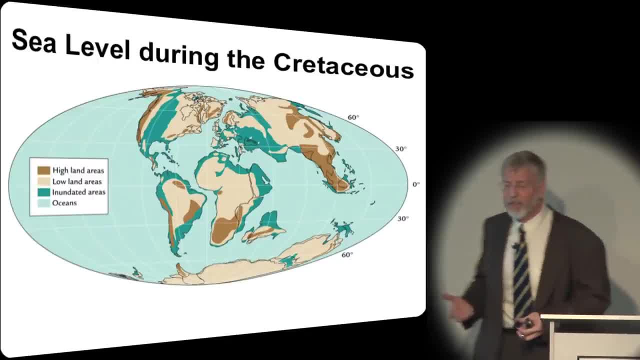 means a much higher sea level, Something like 150 to 200 meters higher sea level. So the downside is that St Louis is a seaport. So the downside is that St Louis is a seaport. There is no fault. 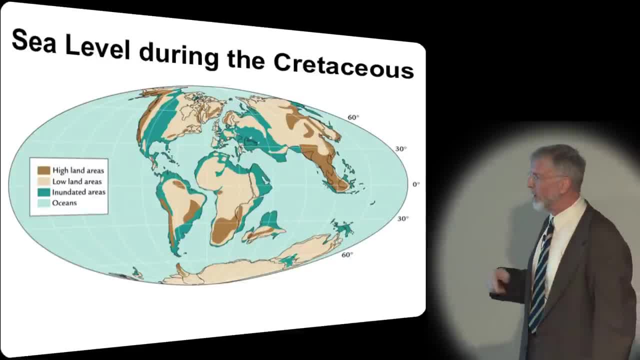 Florida above the waves. All of Florida is part of a shallow sea. Almost all the coastal areas are inundated. The Middle East is mostly underwater. So there are good parts and bad parts, like anything else. So it's much warmer. You can live in Ohio quite pleasantly, except. 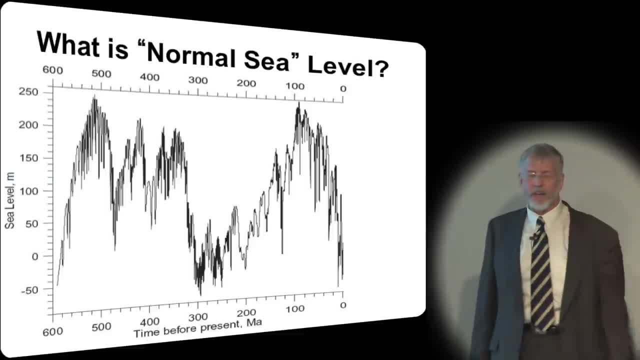 you just don't get to live in Florida. Now you ask: well, is that normal? Well, what is normal sea level? We are here at zero. If any of you work in the oil industry, you might recognize what is called a veil curve. This came out of the oil industry after spending. 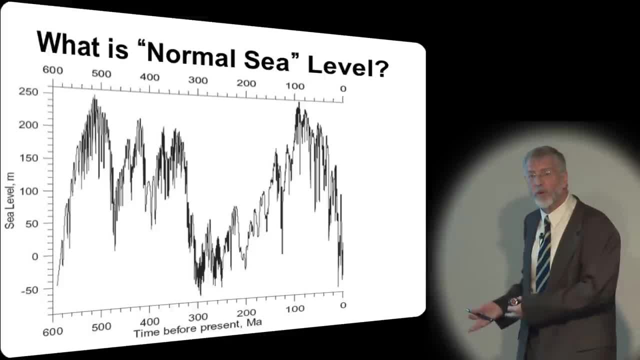 literally billions of dollars of research, because this is how you find oil. The way you get oil is what geologists call a succession of transgressions and regressions of sea level Which trap the right sort of critters and right sort of sediment underneath the right 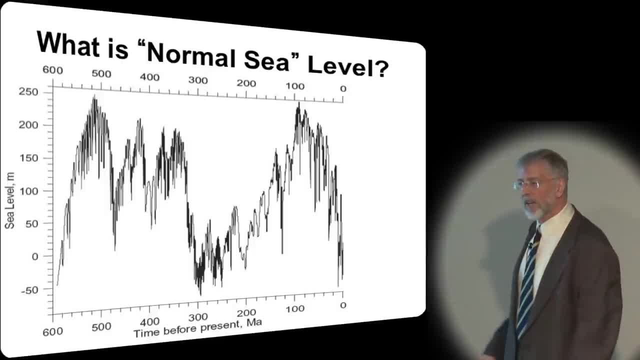 sort of layers of stuff in order to make oil, And that's very much a function of sea level. So this is actually pretty damn good data, Because you know you make billions and billions of dollars, if it's exact. So that's a good reason. It's not just because, hey, you get. 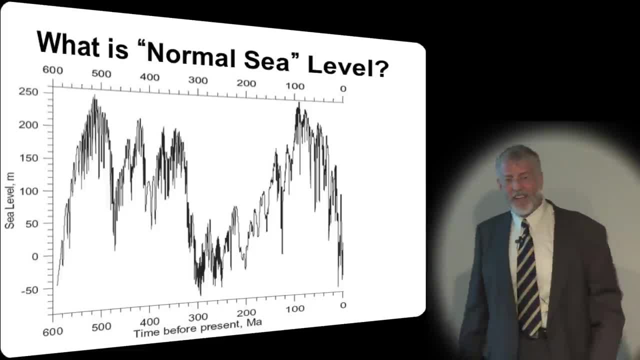 tenure or something. You make vast amounts of money And they fire you if you screw up, And yeah so, and also you see the spikiness here. That's actually real. Sea level is actually highly variable, and not just from melting glaciers. It turns out that the mid-ocean 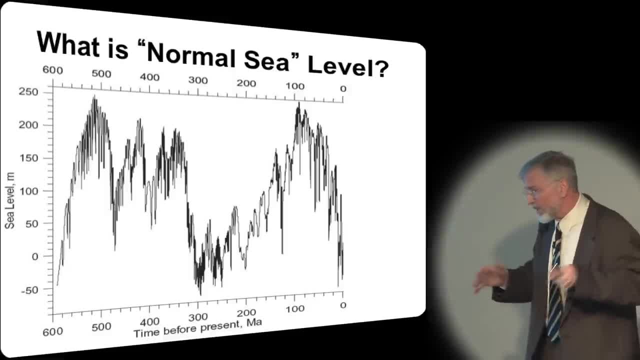 ridges where most of the volcanism occurs. this plate tectonic stuff, the plates actually move around. they actually vary quite a bit And when the, when the mid-ocean ridges decide to crank up and expand and create plate faster, they actually expand. If they expand, there's 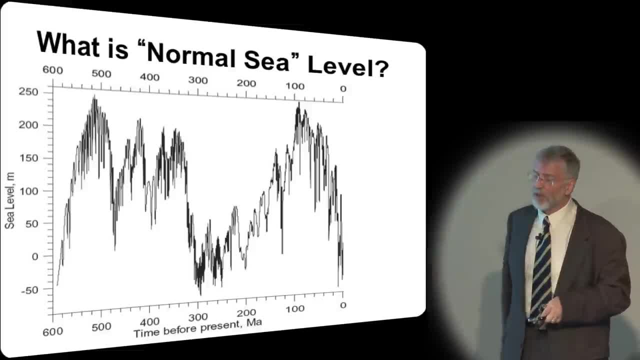 no other place for the water to go except into your homes and gardens. So, and this occurs on, you know this is geologic time again, So it occurs on like million year timescale. So you know, don't go out and sell your waterfront property. But you know this is, you have to. 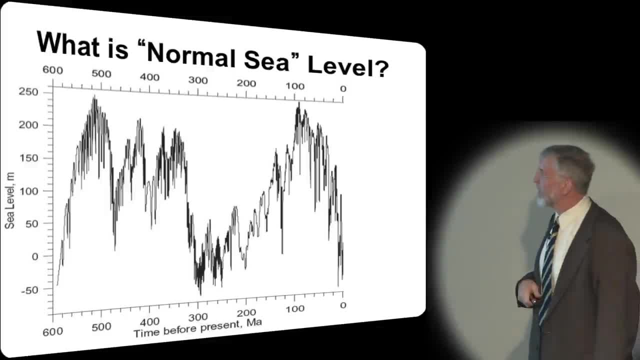 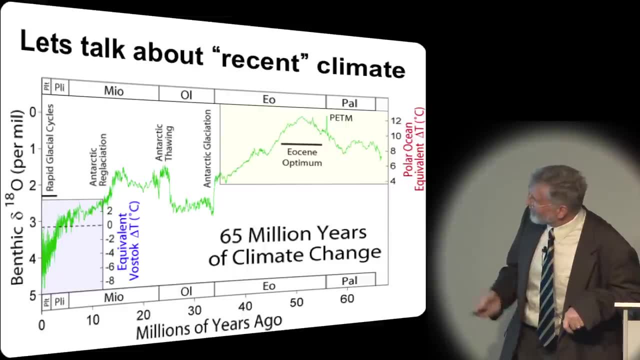 recognize that this is the sort of thing that happens. So let's talk about the recent climate. you know, and the recent climate is like the last 50 million years or so: Back in the Yusin it was pretty warm, And then what's been happening over the last 50 million years is a slow. 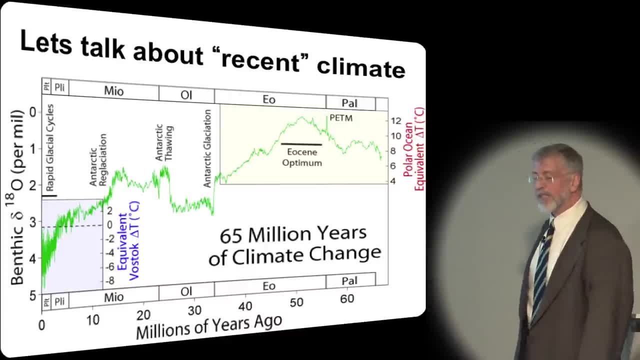 deterioration, but steady deterioration of the climate. You actually, you actually didn't get Antarctic glaciation until about 35 million years ago And then it glaciated and thawed out and re-glaciated And since it's been re-glaciated over the last about 12 million. 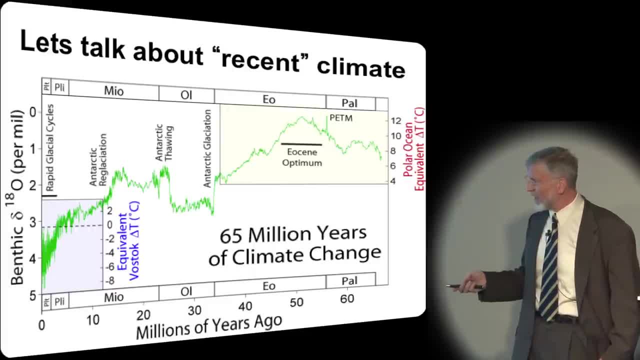 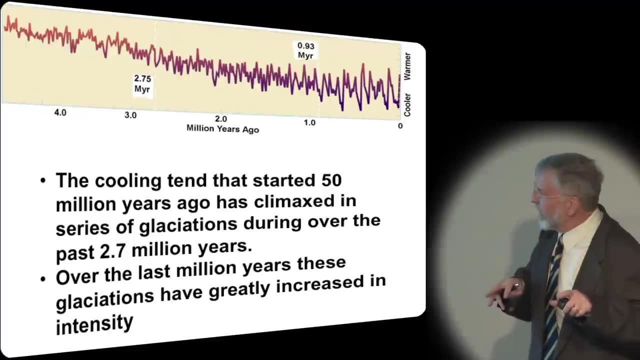 years there's this been this very steady, very short-lived, very short-lived, very short-lived sharp drop in the average temperature of the globe. Why is this happening? Well, before I go into that, I just want to say that this: if you just look at the last 5 million years, this trend is 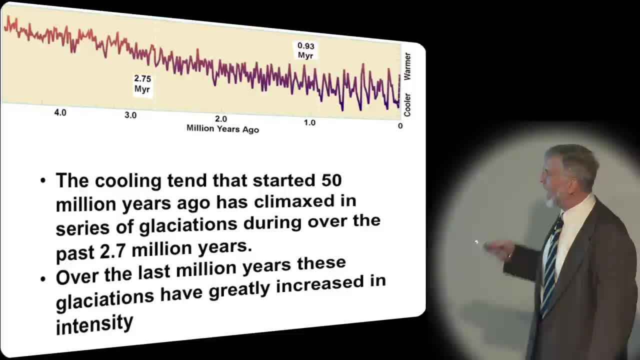 continuing. It's been very steady, And what happens is that it's climaxed in a series of glaciations, And the last 5 million years, these glaciations have greatly intensified, And so you're getting bigger swings in climate as it gets colder, And so what we're we're living in is a relatively 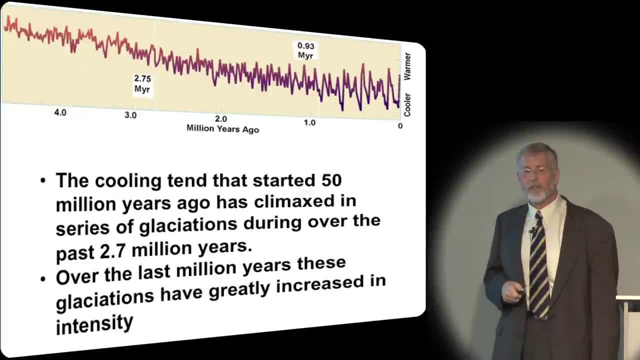 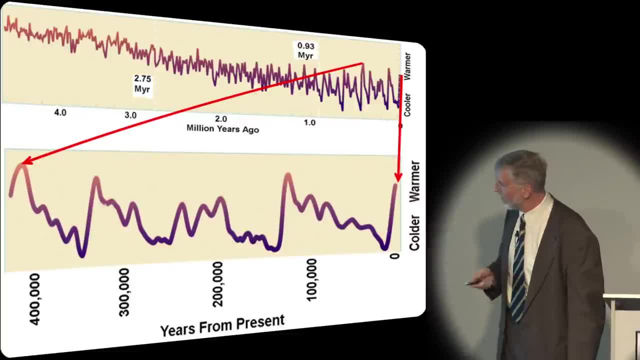 warm period of what is an incredibly cold period in Earth history. So this is the last 400,000 years And I actually took some of this data. We are here And what you find is, for the last 400,000 years, there have only been four periods when it. 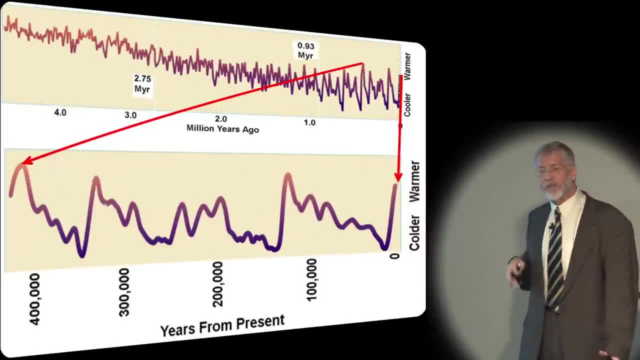 was this warm, And these periods usually last 3,000 or 4,000 years. Does that make you worried? It made me worried when I took this data. It's okay, though, I'll show you why, But anyway we're. 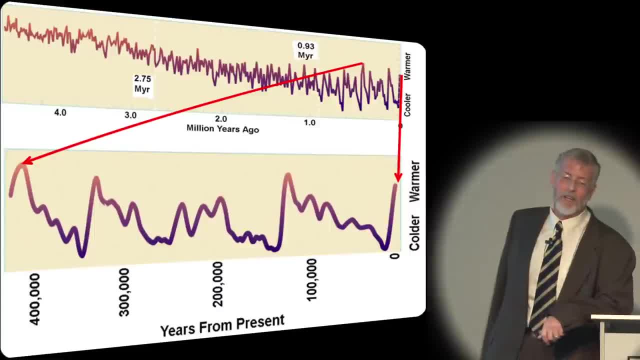 here and we're actually in the most extraordinary long interglacial. This is. these are the warm periods, are called interglacials, And these things are typical. the glacial periods are characterized by the stepwise deterioration in climate down to a glacial maximum. Now, what are glacial maximums like? 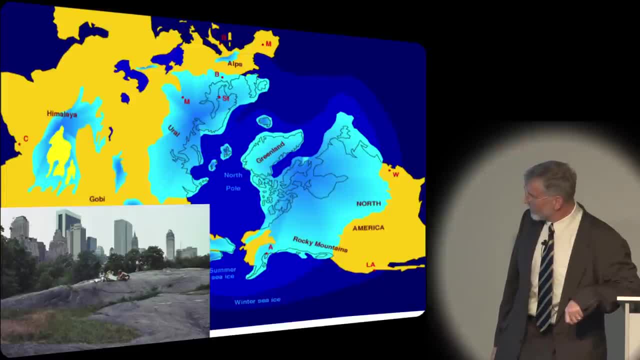 The last glacial maximum was 18,000 years ago. Last glacial maximum: you had a mile-thick glacier, mile-thick ice. in New York City, Berlin and London. You had a mile of ice. over Seattle. You had continuous sea ice down to Cape Hatteras. 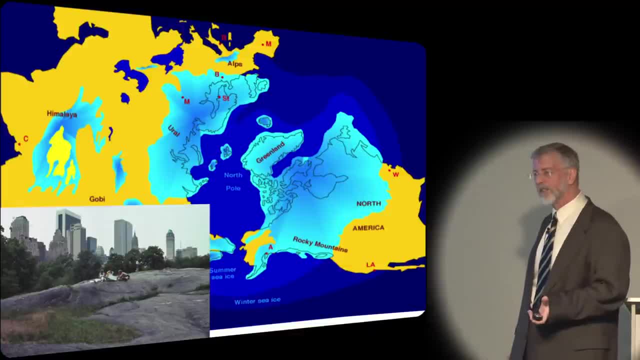 in the winter. Can you imagine your condo in Cape Hatteras in the winter with continuous sea ice, Continuous sea ice down to Baja California? Well, I've been to Baja California. I've gone in the ocean. there It's cold. I can see why it would have. 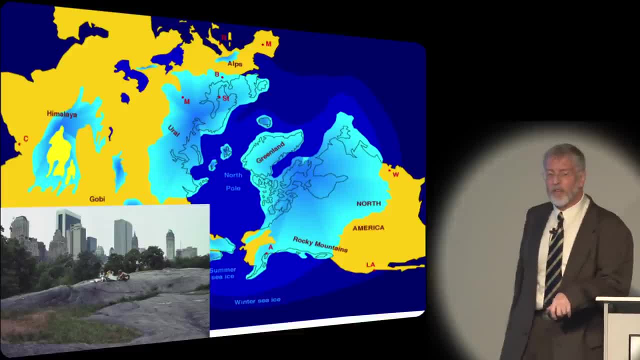 sea ice there, but still, That is kind of extreme, But we have excellent geologic evidence that that's what happened And you had continuous summer sea ice all the way along the continents. How do we know this? Well, once again, you can go look at the. you can read this out of the geologic record. You can look for what are called. 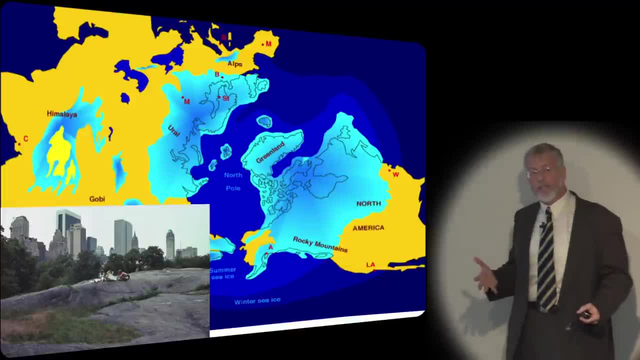 geologic striations. And don't believe me, Go and look for yourself. This particular location is the bedrock in Central Park and you can see grooves cut in it. from the rocks dragged on the bottom of the glacier, You can figure out how thick and what. 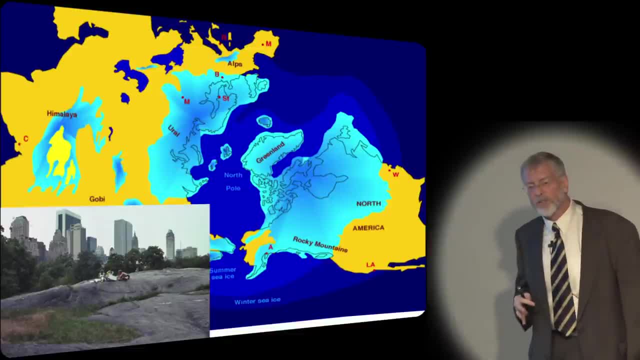 direction. the glacier was moving from the depth of the grooves. This particular one is across the street from the American Museum of Natural History. As you go through the Iron Gate, turn to the right, Go and look for yourself. Same thing with the crocodile turtle and breadfruit fossils in the Canadian Arctic. You can go to these fossil. 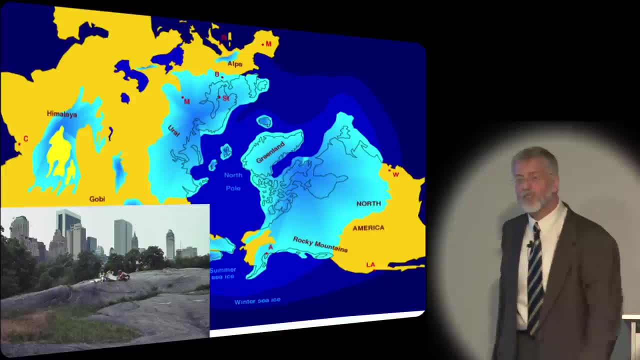 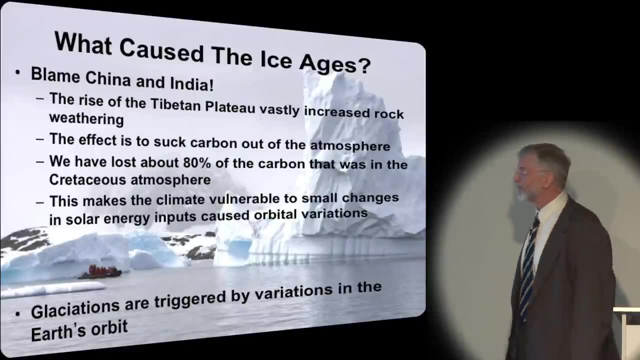 locations and you can look for yourself. I urge you to do that: Watch out for the polar bears. So what caused the ice age? Well, blame China and India. Seriously, What's happened is that we actually live in an extraordinary- I keep saying this- we live in an extraordinary time in earth history, but we do. 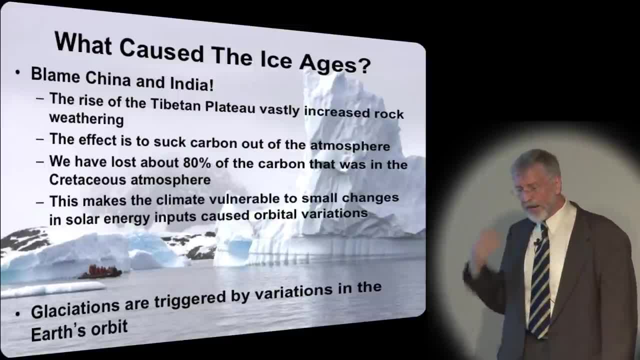 Very few times in earth history are you able to walk to the bottom of the stratosphere on a mountain, But you can do that in the Himalayas. That is a very rare event. You think, because you can do it today, that it must be normal for earth. but no, that's very abnormal. You look back on the geologic 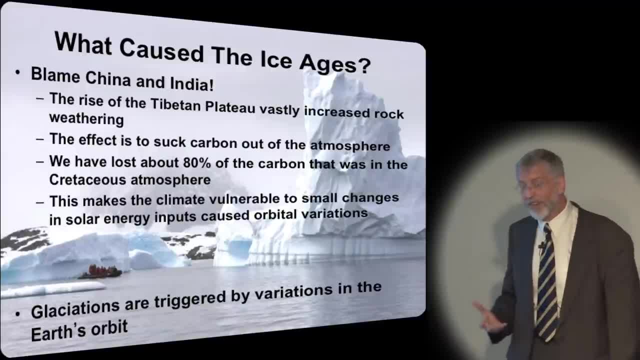 record, and you don't get 30,000 foot tall mountains very often. This is really unusual And what happened is, over the last 20 or 30 million years, India collided with China and created the Tibetan Plateau, an extraordinarily high set of mountains. That really, when you. 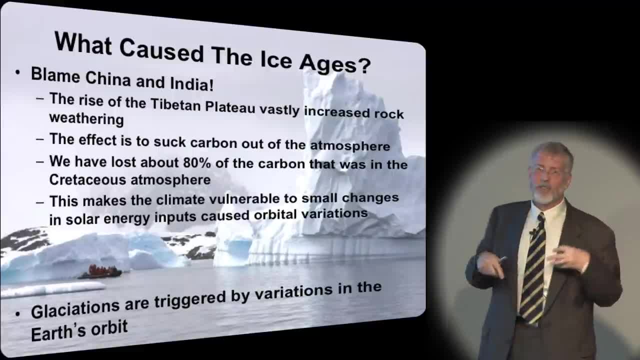 raise stuff up like that and you break up rock like that, what you do is you vastly increase rock weathering. Now I can go into excruciating detail again on the chemistry of rock weathering, but the bottom line is that it sucks carbon out of the atmosphere. 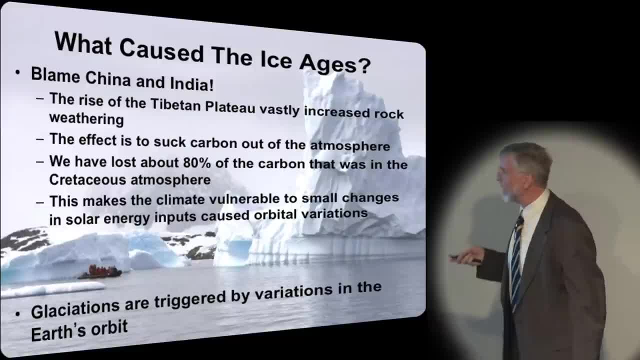 like crazy, And that's what happened here. We've lost about 80% of the carbon that was in the Cretaceous atmosphere due to the Himalayan rock weathering, So you can blame China and India, And what happened was this has basically made the climate vulnerable to small changes. 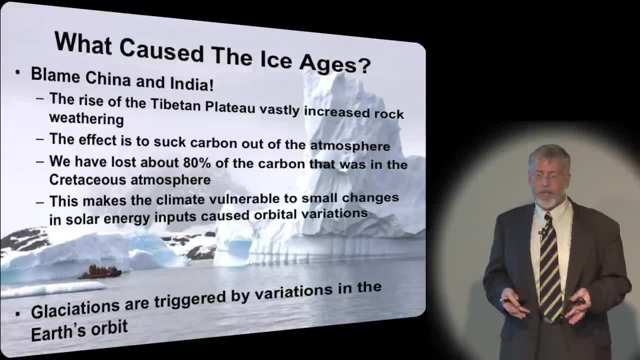 of climate In solar energy inputs Now, and these small changes are caused by orbital variations. The orbital variations are always there, But since you don't have as much greenhouse gas in the atmosphere, it makes it more difficult to distribute heat across the planet. And 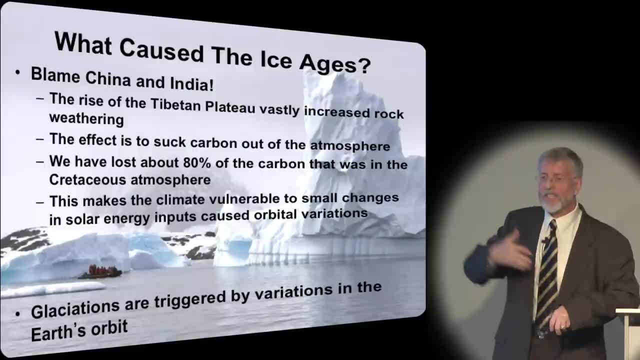 if you don't have the greenhouse gases, you're not going to distribute the heat into the polar regions, And if you drop the solar input to the polar regions, you're going to end up giddy. You're going to end up getting glaciers, And so what happens is that the glaciers are. 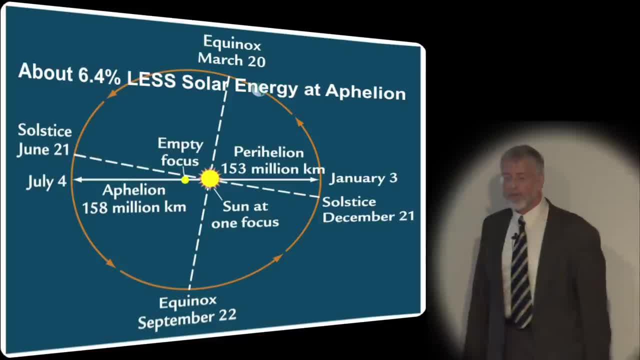 triggered by variations in the Earth's orbit. The way this works is, you know: blame Kepler and Galileo and Copernicus. The Earth's orbit is not a perfect circle. You actually are closer to the sun by about 5 million kilometers in the middle of winter. January 3rd Did. anybody celebrate perihelion on Jan-. no. next year you can celebrate perihelion And it's really easy to remember. aphelion is July 4th. Everybody celebrates aphelion, Nobody celebrates perihelion. I could never understand that. But you get 6% less solar energy at 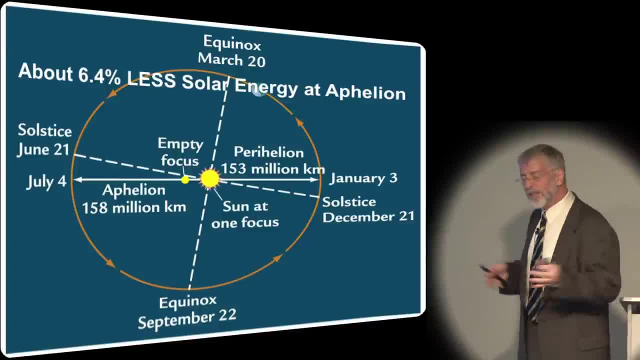 aphelion, And aphelion happens to be in the summer. So the this actually moves around in the orbit and in and in the seasons. It's called precession, And so right now summers are a little bit cooler and warmer. winters are a little bit warmer because of 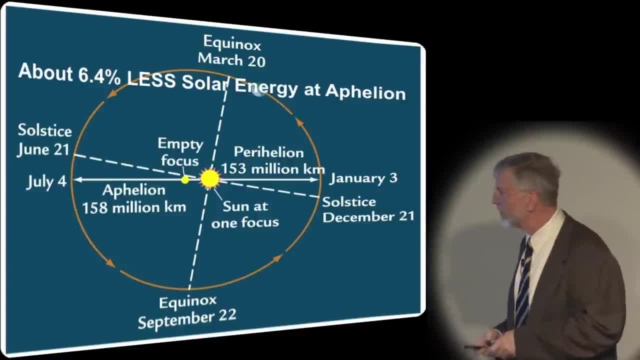 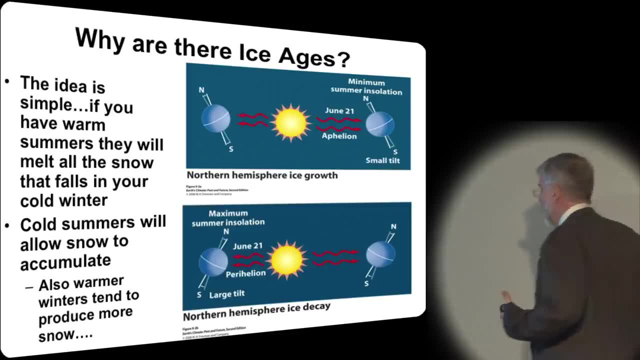 the positions in orbits, But that changes over time And it could be a fair amount. 6% of solar energy is a fair amount. This is basically a simple idea. If you have warm winters, you're going to melt all the snow that falls in your really cold. if you have warm summers, you're going to melt all the snow that falls in your really cold if you have warm. summers, you melt all the snow that falls in your really cold winters. If you have cold summers that can allow snow to accumulate in the right latitude range, And also warmer winters, tend to produce more snow, And I think we're starting to experience. last year was it was a good example of that in the Northeast, where 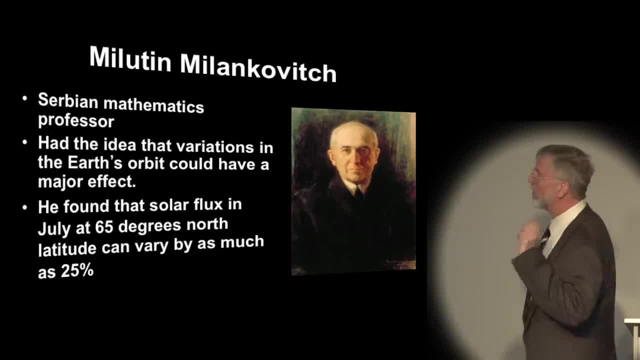 it was relatively warm, but it was really really snowy. The guy who puzzled this all out was a Serbian mathematics professor called Milankovic, And I'm I actually have there's a Serbian graduate student in our group and she just despairs of my pronunciation, So I apologize in advance that I mispronounced. 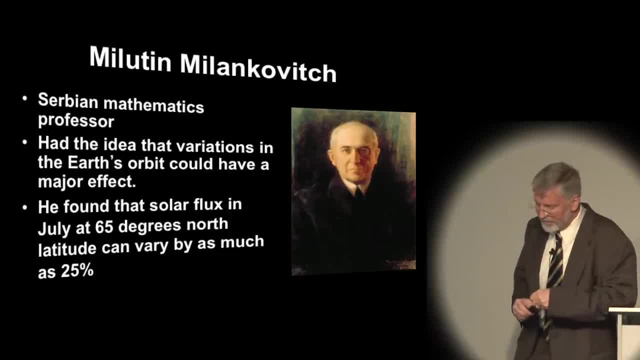 his name. But this is back in the back in the early days of the 19th, the 20th century. this was big science- The question of why there were ice ages, Because you could see abundant geologic evidence that there were at least four big ice ages, four big glaciations in Europe, and 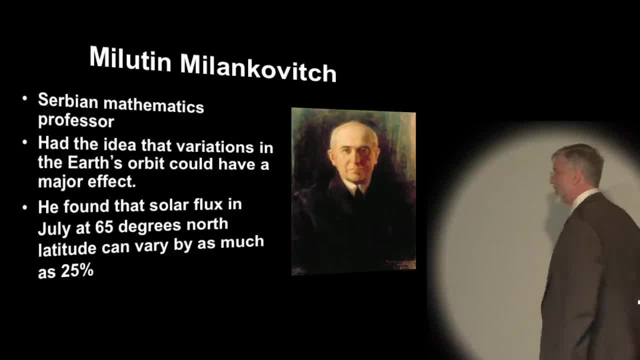 in North America. And and the question, the burning question, was why? And this guy decided that that the way to figure this out was to look at variations in the solar flux at high latitudes, And you can vary that solar flux at 65 degrees north. 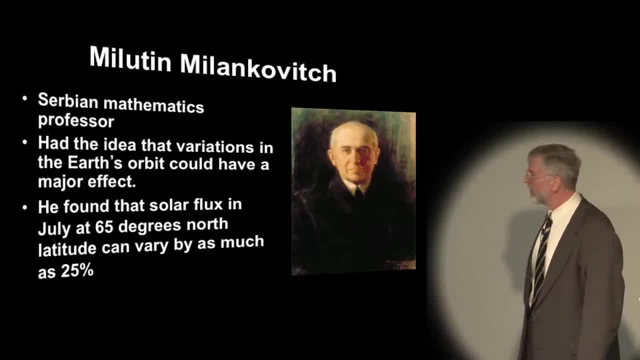 latitude by as much as 25%. But the way to prove this was that you had to do a bunch of spherical trig and figure this out over the last quarter million years. Now a smart student with an Excel spreadsheet can do this in about two weeks Back then. 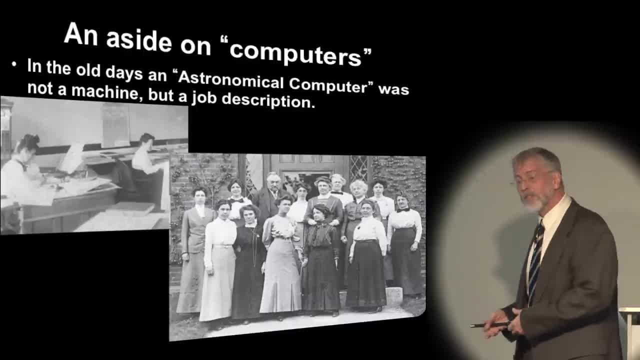 the old days, astronomical computer was not a machine, it was a job description. If you wanted to figure out where to point your telescope, you needed somebody to to puzzle that rule. but inudi- up up over, up you, up, up, up up. 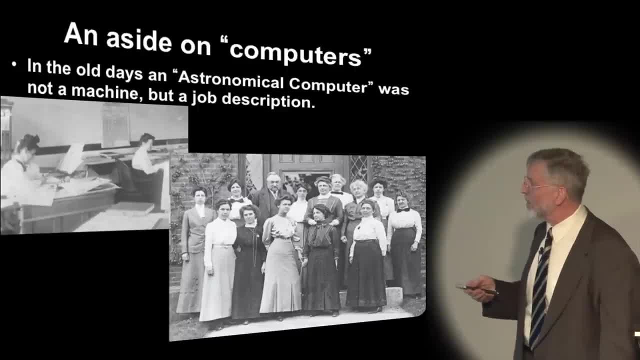 up this out, and so astronomical computers were the people that actually figured that- told the fat bearded white guy who was the astronomer- I can say this, being a fat bearded white guy myself and also astronomer where to do this- and typically the staffs were lots of really smart women who graduated from Ivy League. 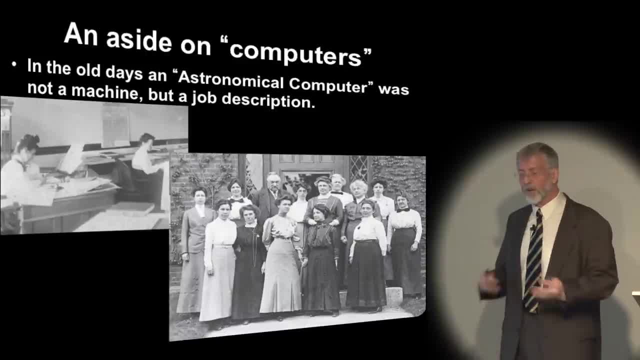 colleges and you know prestigious women's colleges like Holyoke and Bryn Mawr who couldn't get jobs anyplace else. and these guys actually did a lot of the fundamental astronomy in the 19th and 20th century and didn't get any. 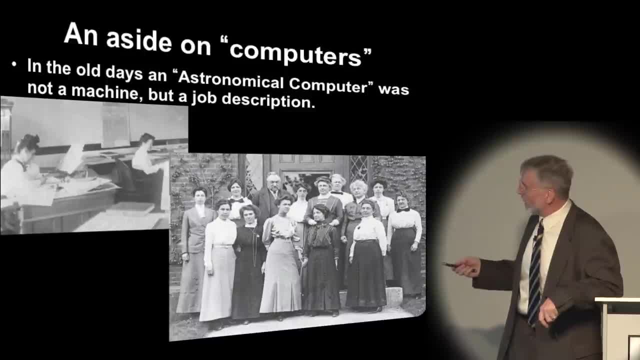 credit for it, because of course this guy wouldn't put any of these names on his papers- a major injustice, being a fat bearded white astronomer. I apologize for that, but that's the way it was. you know the way, the way you figure this out was. 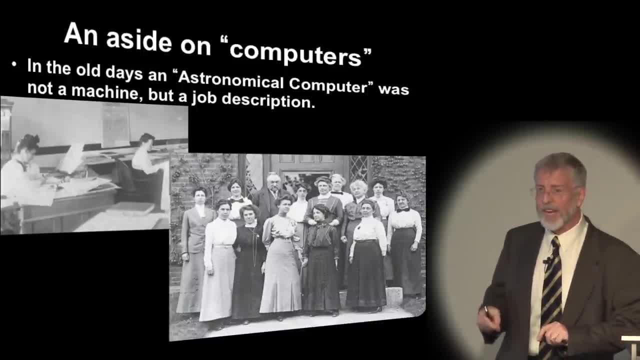 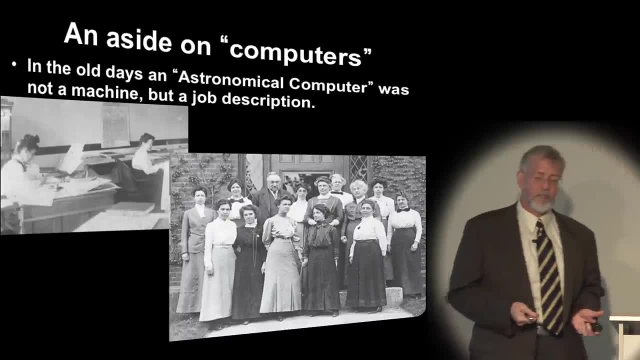 somebody actually sat down and did the math by hand with a pencil, and that's what Milankovitch did in 1910. he started working on this and he figured that if he, his day job was teaching mathematics at the University of Belgrade. and he figured that if he, when he came home and 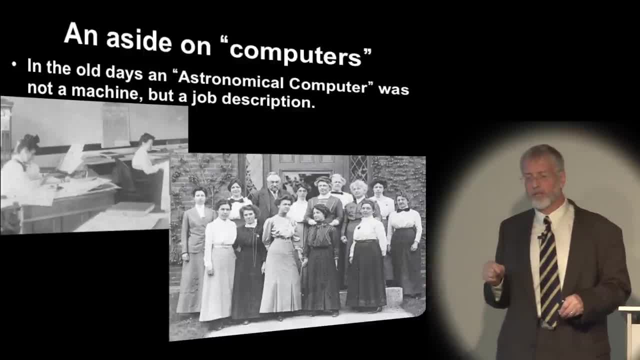 had dinner and then worked for four hours a day, five days a week, and took all Saturday and worked ten hours a day, and then Sunday he would go to church and hang out with his family. And so he did that he could. he could do all the necessary calculations, and only. 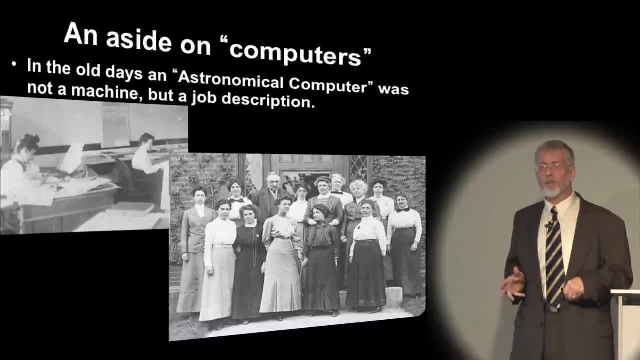 22 years. you know, this was science back in the old days. you know no excel spreadsheets. he well, he was lucky and unlucky at the same time, because what happened was that World War one hit in 1914.. He was a reserve officer in the Serbian Army. he went into the army in 1915 is 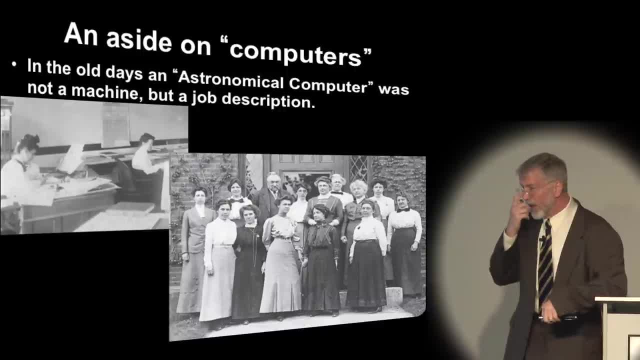 captured by the Austrians, thrown into prison camp and he had a buddy in the in the Hungarian Academy of Sciences who bailed him out of prison camp. and this is a different age. I was an Air Force officer, so I think this is really cool. back in those days, if you were an officer, you could give your word, your parole. 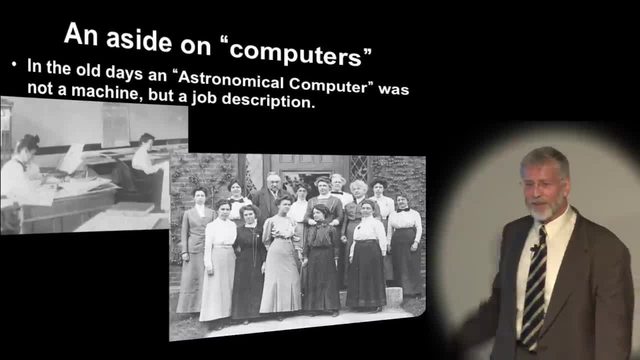 and they would let you out of prison camp and you would promise not to you know. raise your hand and promise not to fight anymore, and then they would let you out of prison camp and you could go off and do your own thing. what a civilized concept. and so what they did was they paroled him to the 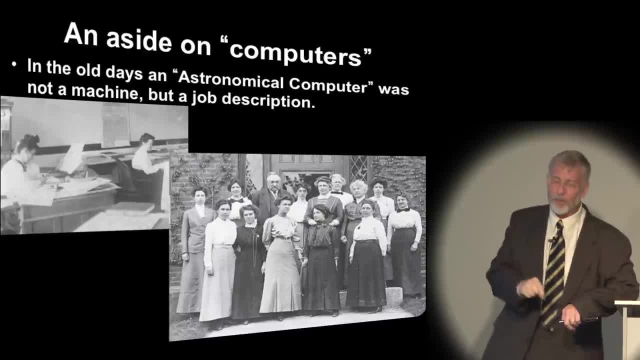 reading room of the Hungarian Academy of Sciences in Budapest for the rest of World War one, and so he was able to work on his stuff ten hours a day, seven days a week, and he actually got years and years of work done during that period and he went back and he actually was able to publish in 1925. 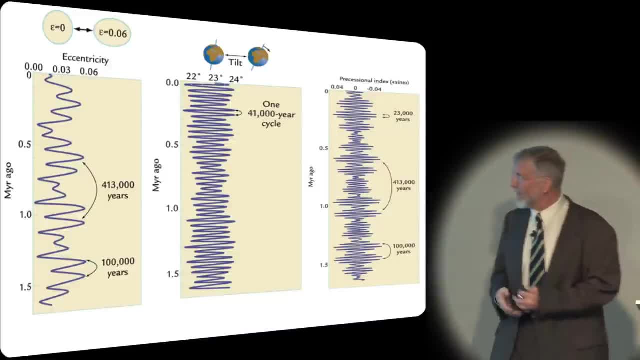 and what he found was that if you look at these cycles, that there's that the orbit of the Earth's orbit actually affects the amount of sunlight you get tremendously because there's the next centricity cycle that goes from about zero to point to six degrees in the in the 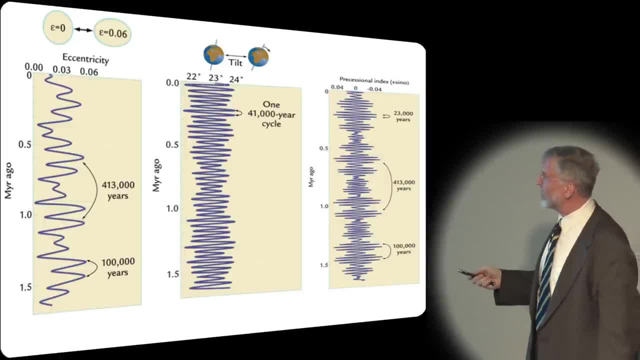 roundness of the orbit. there's a tilt cycle that goes from about 24 to 21 and a half degrees and a, an index of precision, that where you, where you are in the orbit, when you're closest and farthest from the Sun, and you can combine all these effects and actually see how much sunlight you get at high. 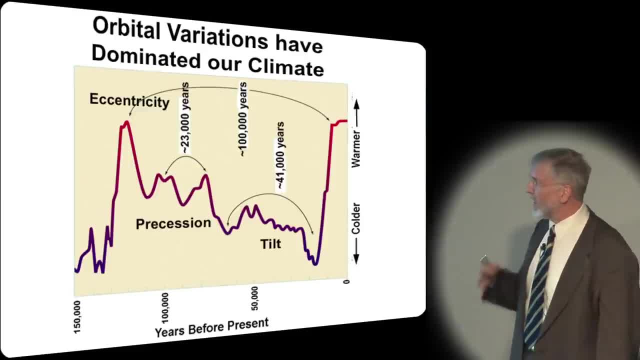 latitudes and it turns out that that just lines up with the relative cold and hot in the climate. this is more of the data that I took, and so there's a hundred thousand year. this is hot, this is cold, this is right now. this is a roughly a hundred thousand years ago. that's the last, that's the previous interglacial. this is the. 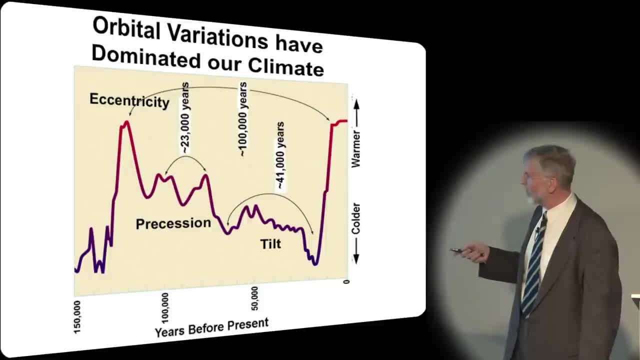 eccentricity cycle: a hundred thousand years. there's the precession cycle: 23,000 years. that's the tilt cycle, 41,000 years it lines up. these orbital changes absolutely dominated our climate for the last half million years and this and all the other things that you see, that you 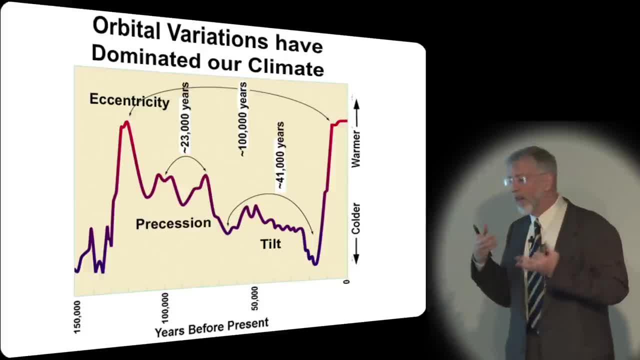 hear about. in climate, they'll need to change. El Ninos, Pacific Oscillations, Atlantic Decadal Oscillations, all these are in the noise, All of that is subsumed in the thickness of the lines you see here, because this absolutely 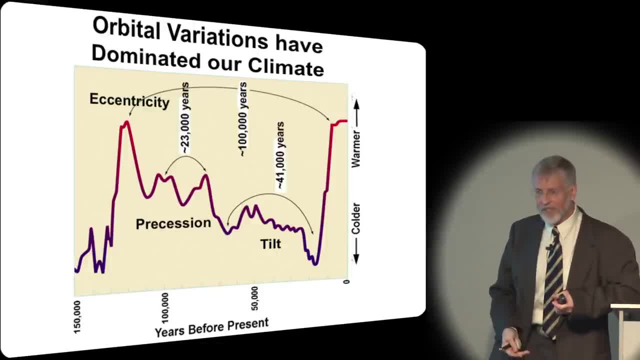 dominates. This is what creates a mile-thick glacier on top of New York City, And just because it's a little rainier- because of El Nino, that's in the noise- compared to having a mile-thick glacier on top of your apartment. 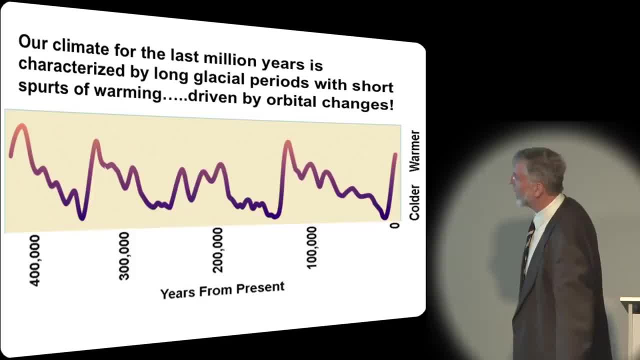 Okay, So that's where we are. So our climate for the last million years has been characterized by these long periods of terrible glacial conditions- Glacial conditions like tundra in southern France. You can go to southern France- I did this last year- and go in and see cave paintings. 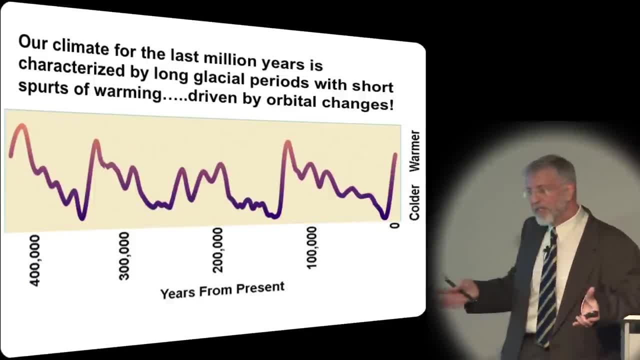 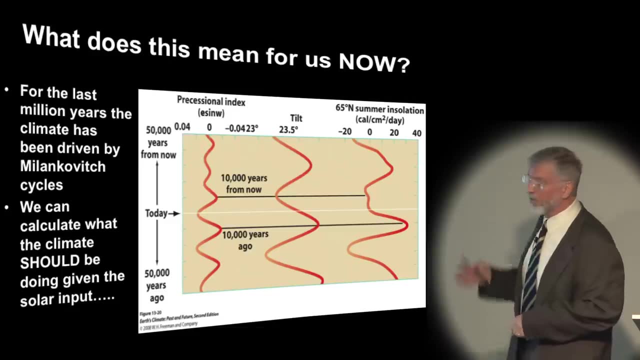 where they have cave paintings of herds of reindeer, because that was the scene. Now you- Okay, You know it's bikini-clad women on the beach, not reindeer anymore. All that is driven by orbital changes, So the nice thing is, though, that you can calculate how these orbits are going to affect. 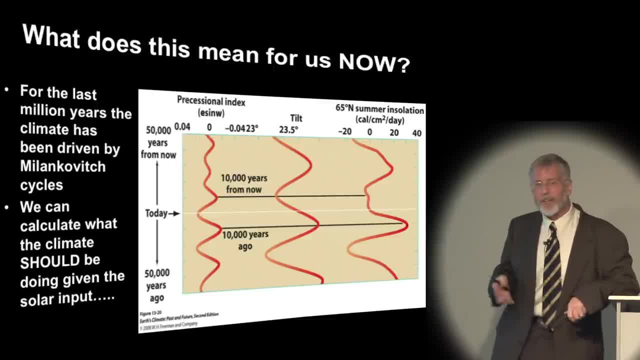 climates, because this is what absolutely has dominated our climate for the last half million years And we should be able to figure out what the climate should be doing, given the solar input, And 10,000 years ago it was really warm. 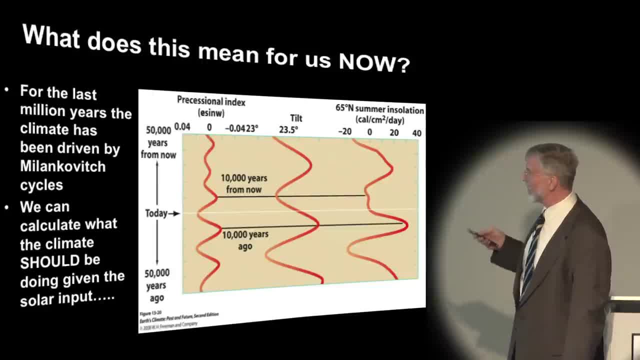 This is the line you need to look at here, because this is summer insulation. the amount of sunlight you're getting at 65 degrees north, And it peaked about 10,000 years ago and then has been in decline ever since. So what should be happening is we should be dropping into the next ice age. 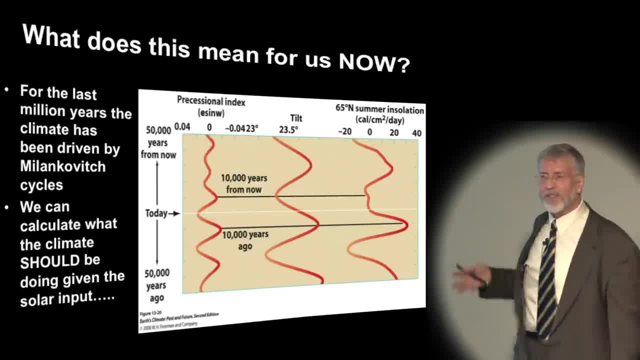 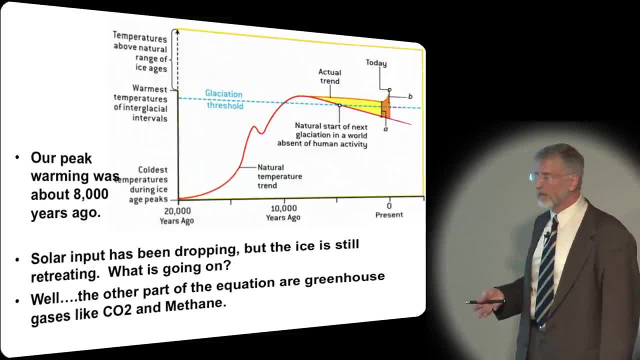 Climate should be deteriorating. Things should be getting colder, given the solar input. Okay, The problem is that it hasn't been. Solar input is dropping, but the ice is melting, So what's going on? And what's going on is us and greenhouse gases- CO2 and methane. 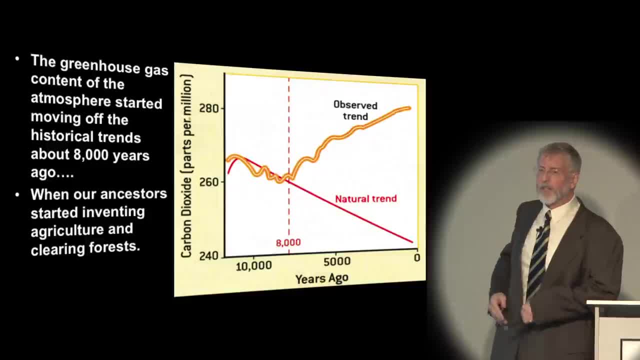 What happened is that our ancestors were smart kids. Up until about 8,000 years ago, The atmosphere stuck with historic trends, But about 8,000 years ago, our ancestors invented agriculture, started clearing forests. When you clear a forest, what you do is you it's slash and burn. 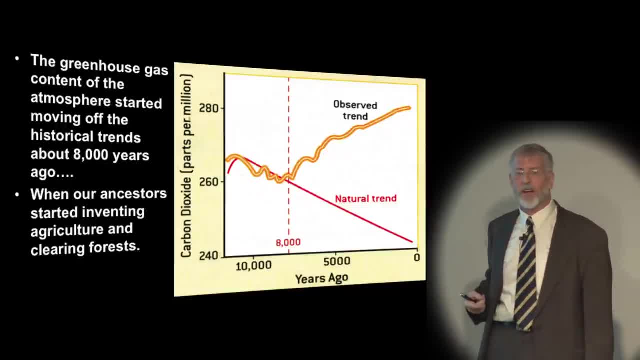 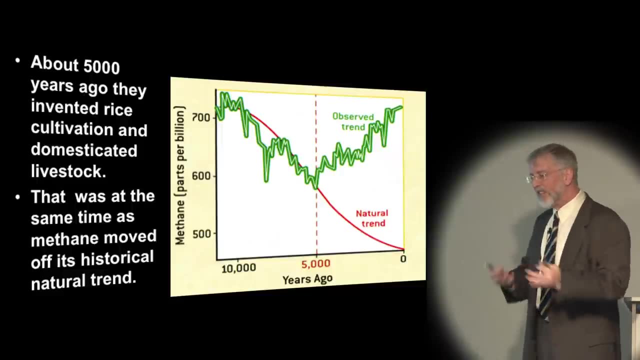 You put lots of carbon back in the atmosphere. You control the forest with fire. Very intensive, very carbon-intensive sorts of agriculture: Methane. the same way, About 5,000 years ago, they invented rice cultivation and domestication. Nothing is a better methane producer than a herd of beef cattle. 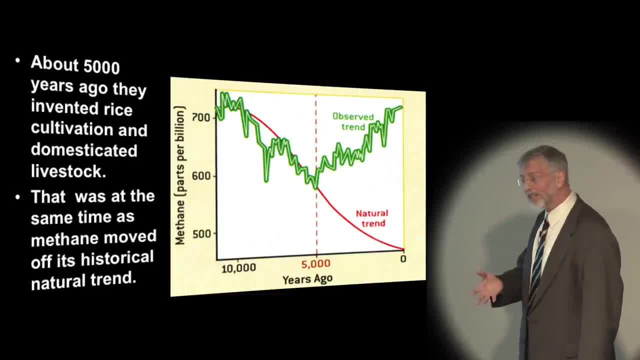 You can also test this for yourself. Go to a cattle ranch. Let me know what you think. The other thing is rice cultivation. I don't know how many of you spend time in rice paddies, But rice is a swamp grass, And so what you need are swamps in order to grow rice. 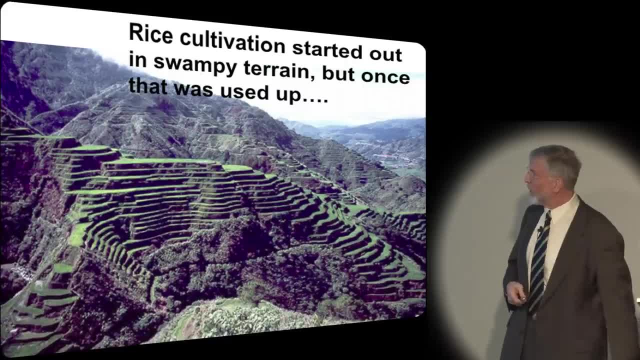 When you don't have swamps, you go create them, and if you it- and one of the tests here is that you can sort of cruise around the Far East on Google Earth just to see how extensive the rice cultivation is- prove for yourself this: these, these terraces are 3,000 years old. 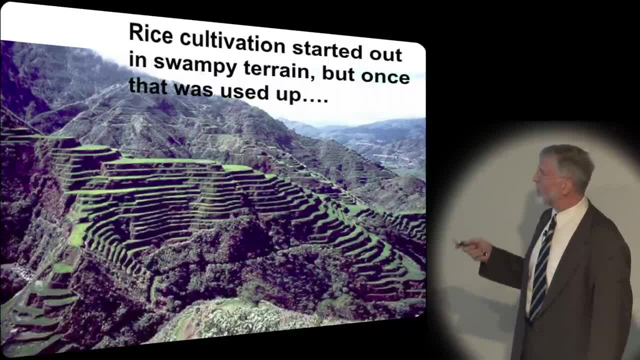 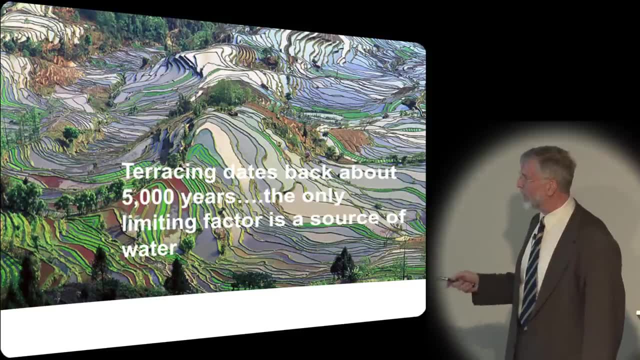 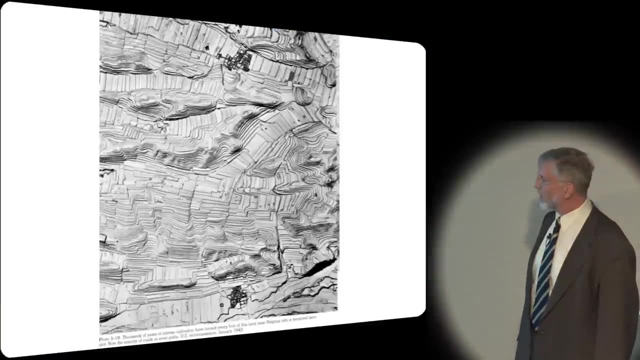 in the Philippines. basically, once you use up the swampy terrain, you got to start terracing or you starve, and terracing dates back about 5,000 years. the limiting factor here is water. if you have a source of water, you can make terraces. I really like this picture because essentially it looks like a topo. 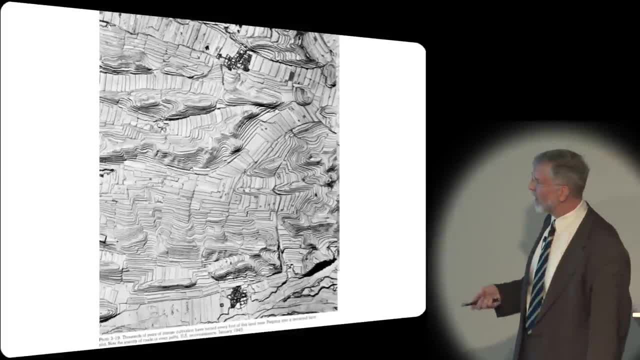 map. but it's not. it's just. this was a book I found in the library. it was done by Claire Chanel, photo reconnaissance officer during the World War two period work for the Flying Tiger, and so he has all these great pictures of China the way it used to be, you know. 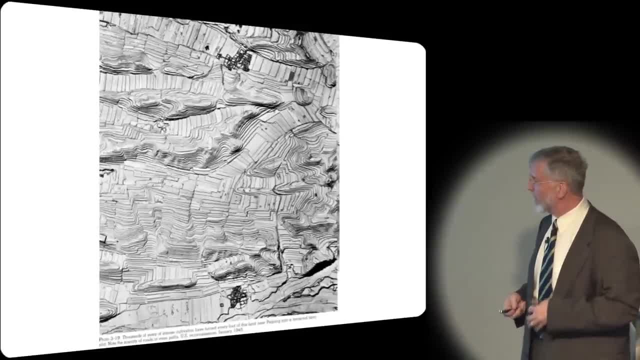 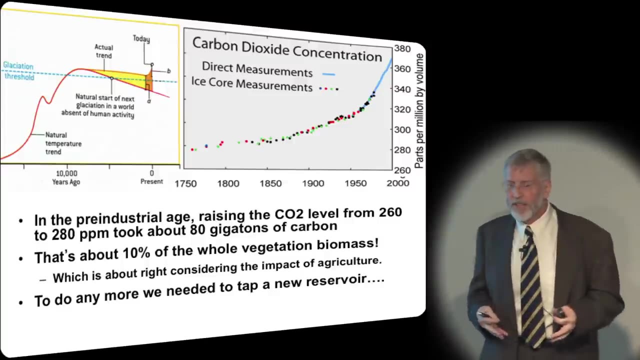 these days they, you know they run superhighways through this, but essentially everything that had a sort, everything that could be terraced, was terraced, and so human input to the atmosphere started a long time ago. it's not just us in the Industrial Age, basically in the pre-industrial age, you. 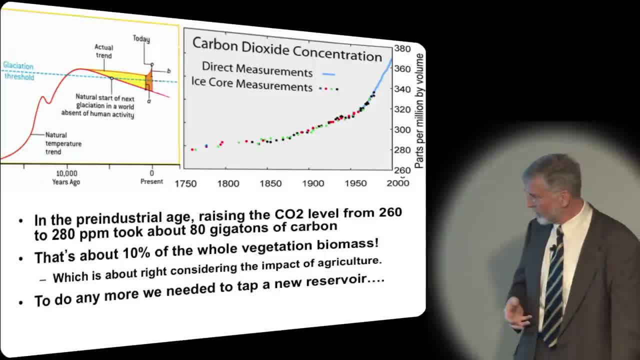 started out with about Parts per million co2, and human activity stop the decline of co2 and and and methane in the atmosphere and cranked it up to about 280 parts per million, essentially putting carbon gigatons, billions of tons of gigatonnes and billions tons of carbon into the. 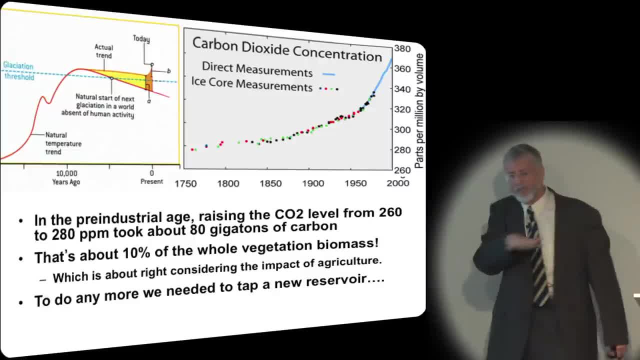 atmosphere. so about 80 gigatons of carbon. that's equivalent to about 10-percent of the biomass. but that's about right for the forest clearing That happened in the pre-industrial age. The problem is that your solar input is still dropping. 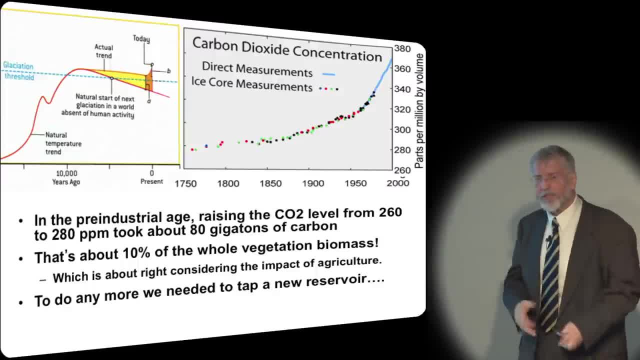 And so, even though you're tossing in more carbon from burning more forests and domesticating more livestock and making more rice paddies, there's a point of diminishing returns. And so, actually, things started to get colder back in the Middle Ages simply because you couldn't keep up. 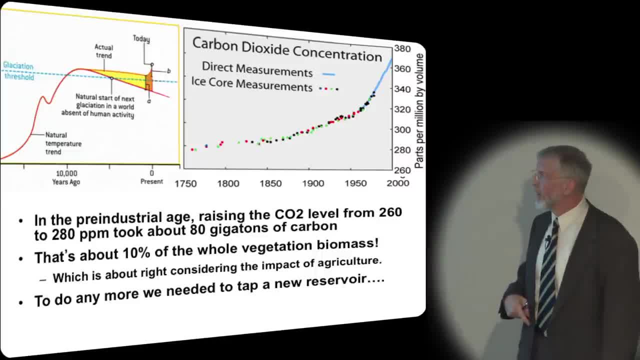 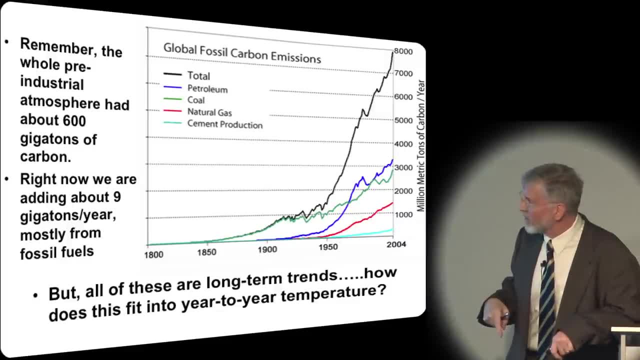 What we did then was we tapped a new reservoir. We figured out how to get into fossil fuels and use those. The whole pre-industrial atmosphere had about 600 gigatons of carbon in it. What we do now is we add about 9 gigatons a year. 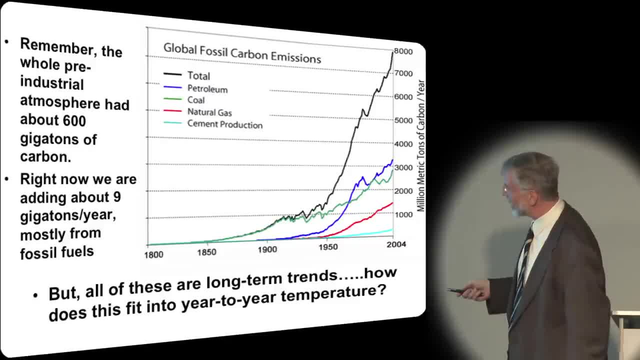 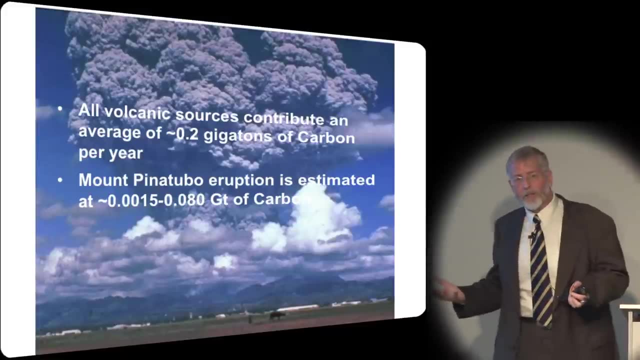 almost all from fossil fuels. There's a tiny little bit. This is cement production right here. All the rest of this is: This is fossil fuels. People say: well, you know what about volcanoes? On average, the entire volcanic input. 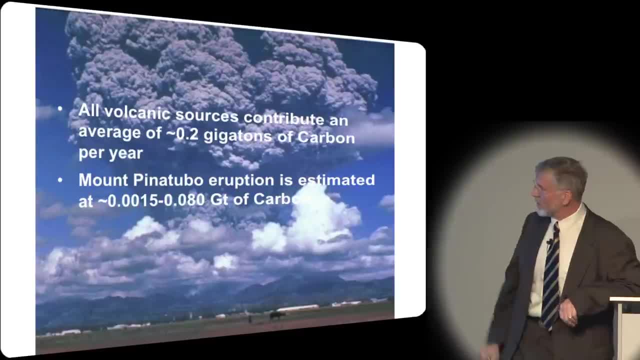 into the atmosphere is two-tenths of a gigaton of carbon per year. People say, well, what about Mount Pinatubo? This is Mount Pinatubo. Notice the guy with the water buffalo plowing, who's ignoring the largest eruption. 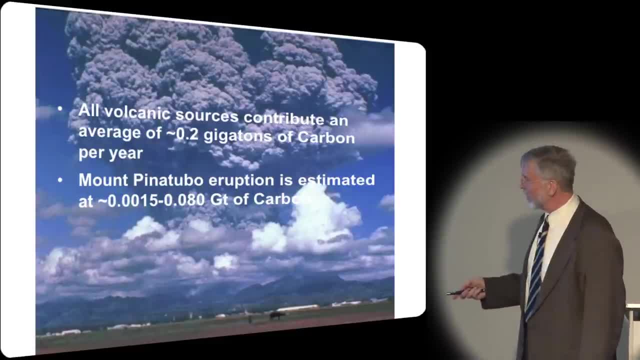 in the last 150 years. That's Clark Field in the background. since this is a flyer town, Probably a few of you have flown into Clark Field. Clark Field was a little bit the worst for wear after this, But anyway, the Mount Pinatubo eruption, they're not really sure. but this is in the noise. 0.08 gigatons of carbon is the maximum estimate. That's in the noise. The biggest natural input- net input- to the atmosphere is volcanism, And that's 45 times lower than the human input from fossil fuels. 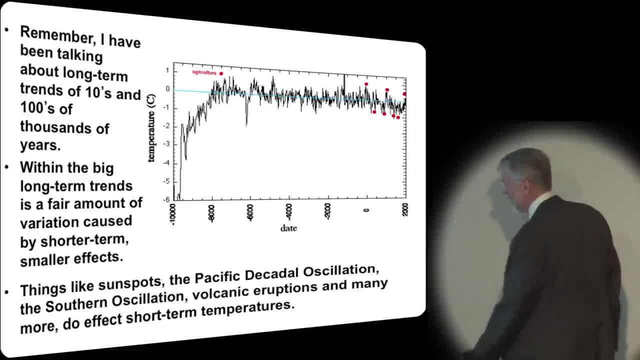 every year 45 times. Now, remember I've been talking thousands of years in hundreds of thousands of years. These are big trends. scales: you and I live at human scales, And so year-to-year variation, or decadal variation, means a lot. Within the big trends, there are a: 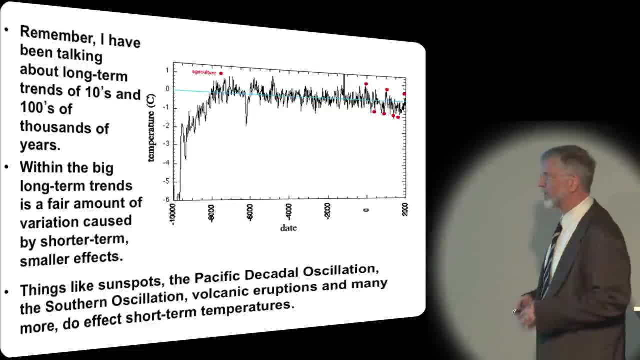 lot of short-term effects, Things like sunspots, Pacific decadal oscillations, southern oscillation, volcanic eruptions, all sorts of other things too, And all of these have an effect on short-term climate, because this spikiness is real. 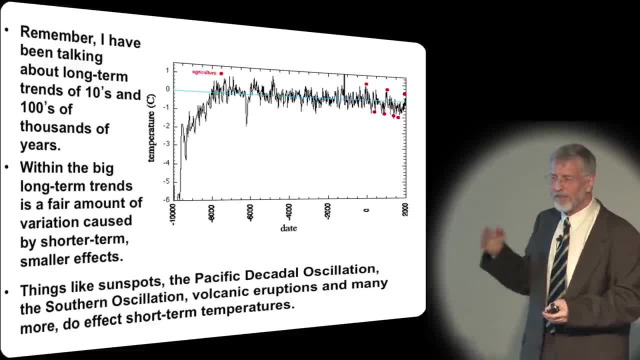 That's the noise that I said was the noise I was talking about in these big swings. But remember, when we're talking about big swings, this is a swing down into the Ice Age. It goes about another six degrees down here. So that's what I'm talking about with the 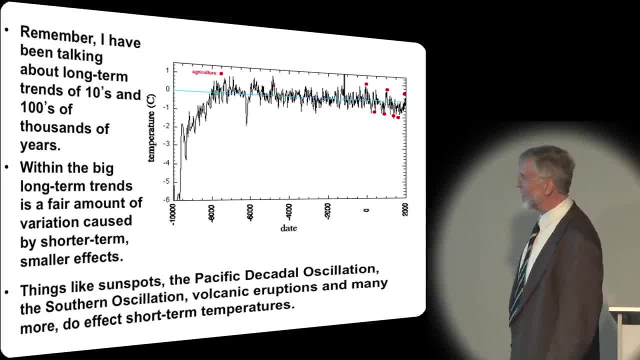 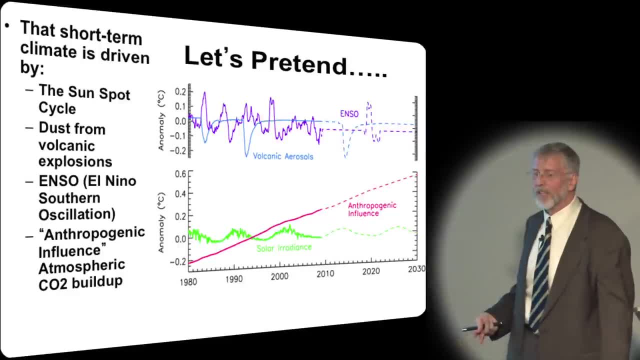 big glacial swings. So we live up here in the spiky area. Let's pretend, and I don't like to do climate modeling because that's really complicated. I like this model because it's fairly simple. I'll just show you this to show that it's possible to explain short-term. 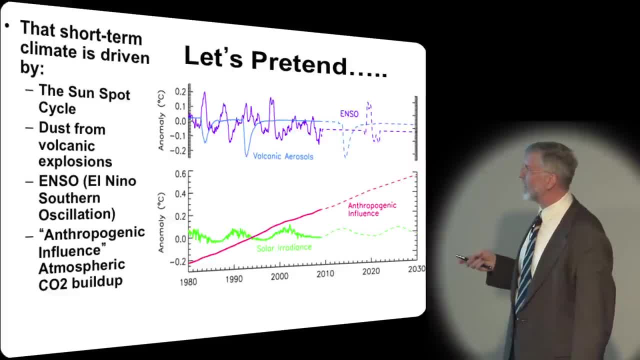 variation. Let's pretend that short-term climate is driven by four things: The sunspot cycle, because sunspots do affect solar irradiance and the amount of watts per square meter that the sun dumps on the Earth. So you get an 11-year cycle where you get a little more. 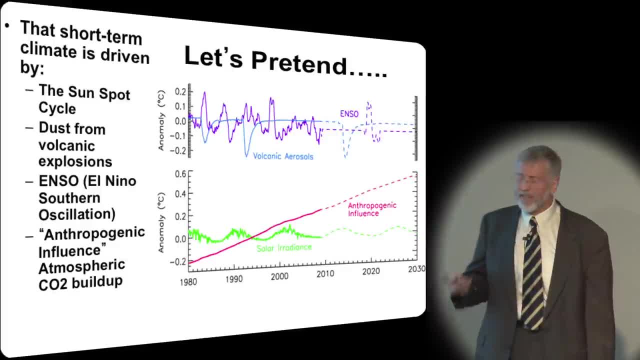 irradiance and a little less, and it affects it on the order of less than a tenth of a degree C, like half a tenth of a degree C. Then you get volcanic aerosols. Mount Pinatubo blew up and threw a lot of gunk into the upper atmosphere and that actually cooled things. 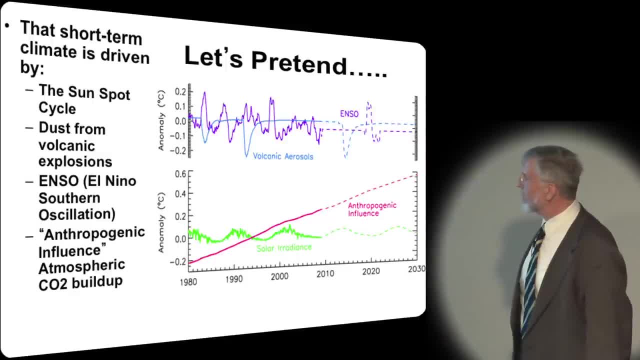 down quite a bit, That's Mount Pinatubo right there. Then you get the El Nino Southern Oscillation. El Nino actually does change the energy balance because it's a big lump of warm water that sloshes around the Pacific in the simplest. 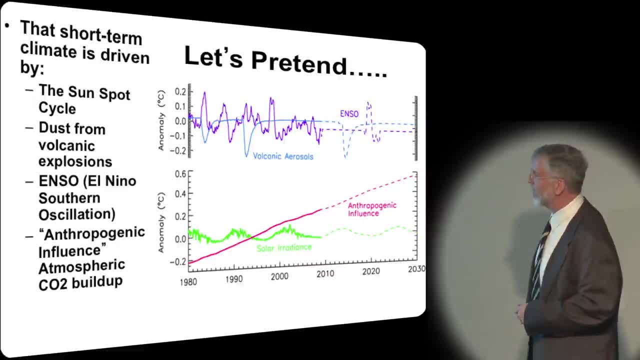 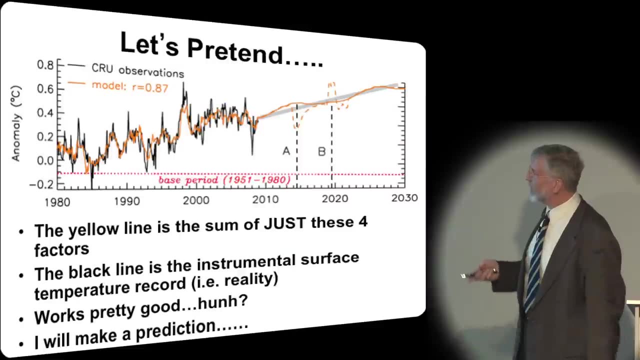 sense. Once again, we can do this more complicated. But if you sum all of these things and say that's what drives the short-term climate, with this anthropogenic influence that is, dumping more carbon in the atmosphere, You can actually model the black line as the instrumental surface temperature record. 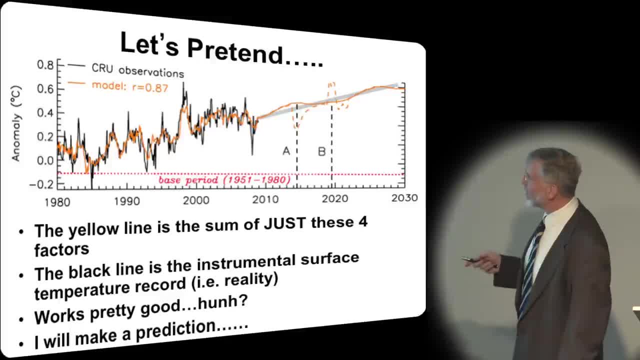 or, as I like to call it, reality. You can actually model reality pretty damn well. Not bad, though, Fit is 87.. The thing is, though, that we're just coming out of a very low sunspot cycle, Actually in the last 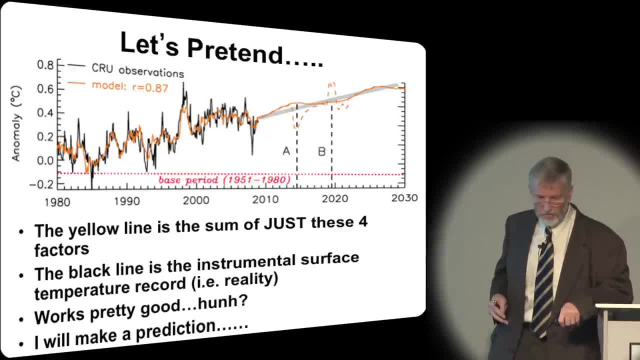 50 or 60 years, a historically low sunspot cycle. Things were actually slightly cooler because of low sunspots, but we're going into solar maximum right now. Sunspot cycle is cranking up. As a result, what's going to happen, I will predict, is for the next four. 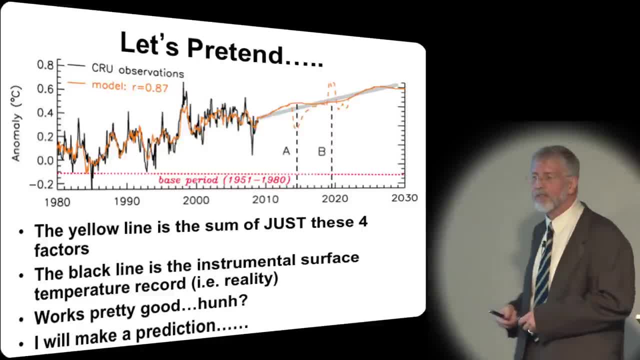 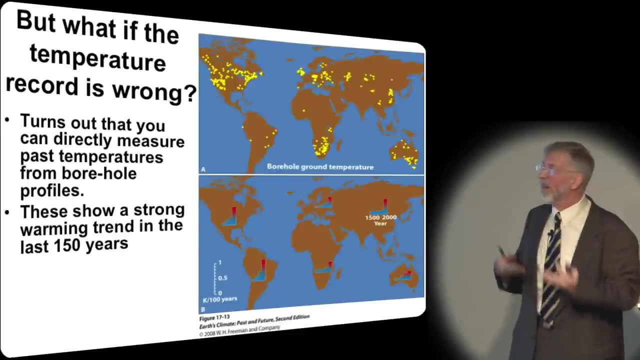 or five years, you're going to have a succession of extremely hot years. Sad but true. So far it's proven. The average temperature records have been proven to be very, very low. It's been proven that that's, that's what's happening. So of course people say, Well, is the? 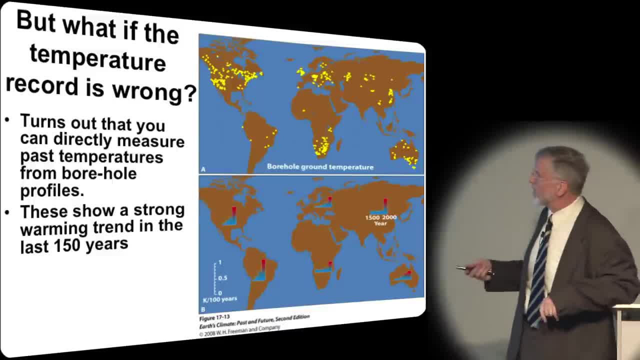 temperature record wrong? Well, it could be, But it turns out that you can. you don't have to rely on instrumental records. you can do things like. you can measure temperatures directly from bore holes, Because there's actually a temperature record that's preserved in the in the 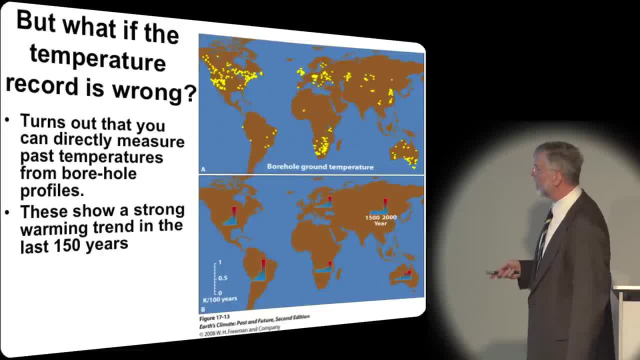 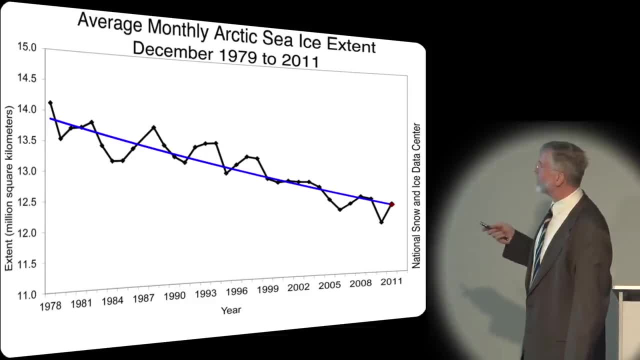 the, the shallow crust- All of these show strong warming in the last 100 years. You can measure. You can look at the average monthly sea ice extent. This is updated to this year and it's declining. You can look at Alaska growing seasons that are getting progressively longer. 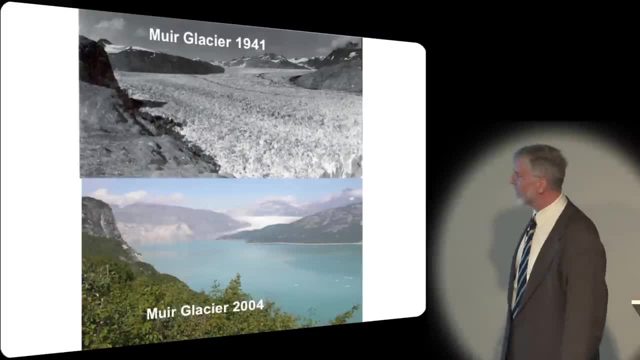 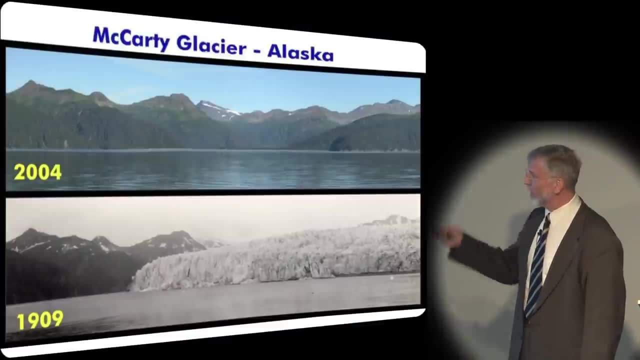 You can look at low elevation glaciers in Alaska. The one I showed you was Muir Glacier. That's not the only one- McCarthy Glacier. I love these guys because what they did was that they went through and got a whole bunch of old National Geographic style pictures of glaciers in lowland Alaska and then went. 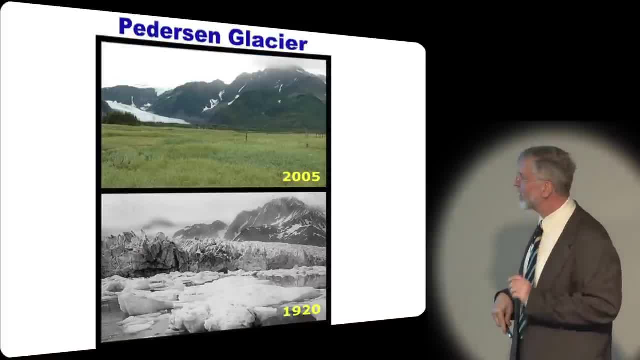 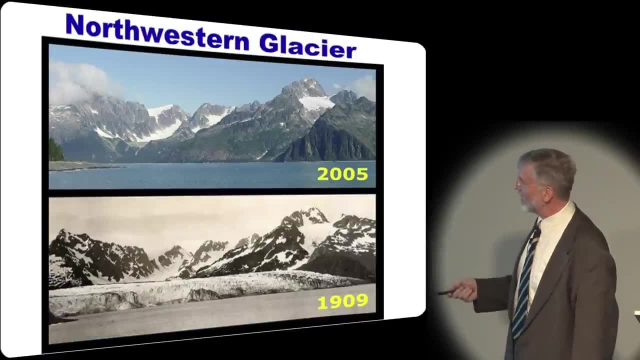 to the exact same place and took another picture. I love this and I've got a big collection. I'll bore you with a few of them, because I just love these things. Northwest Glacier- Northwest Glacier- really got hammered There. it is way back up there. 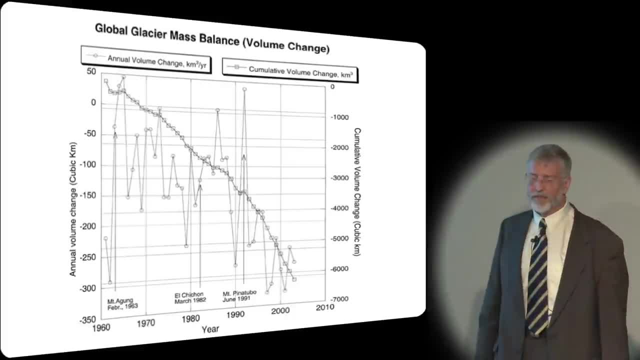 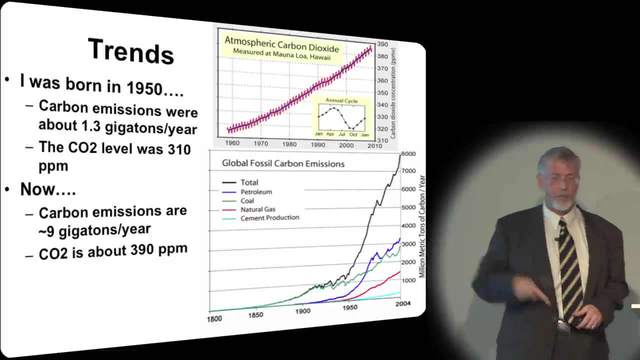 Point is that you can look at a glacial mass balance and it's just dropping off a cliff. It's a big one. I think it's called Herring Field. Those are the big ones. This is a kind of the great Great. 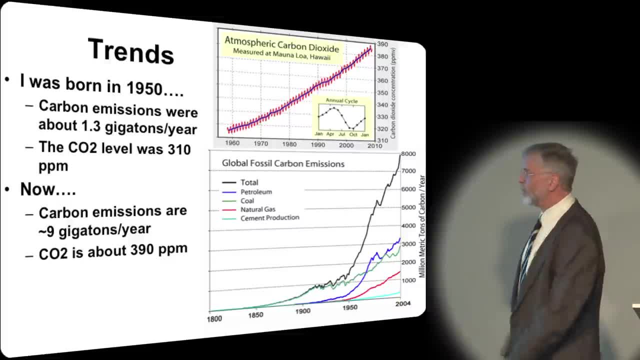 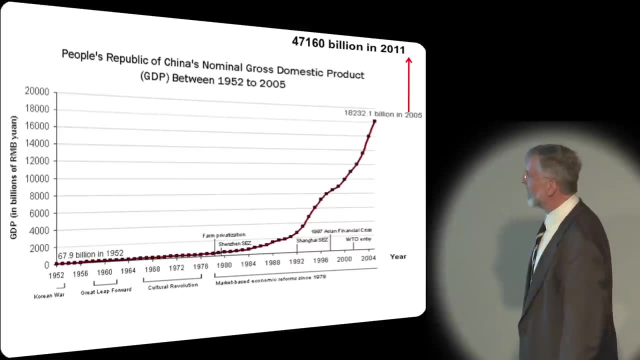 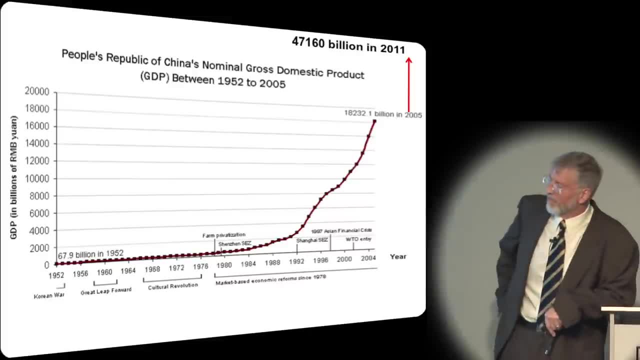 went to graduate school, I was in my mid-30s, And so when I walked into Brown University, I was the oldest graduate student at Brown University. I ended up sitting next to a guy who was the second oldest graduate student at Brown University: I was 35, he was 34.. 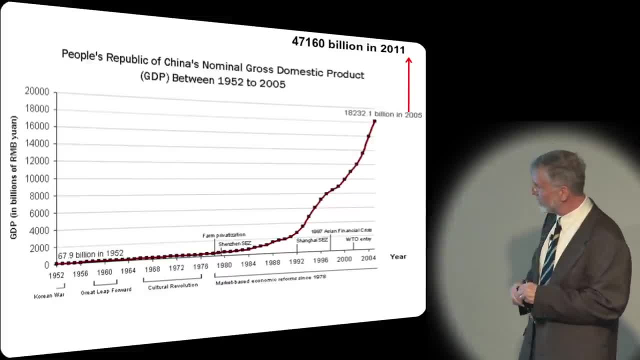 A guy named Wei Deng from People's Republic of China. I said, Wei, you know 34, that's pretty damn old for a Chinese graduate student. And he said, well, yeah, I went to graduate school back in the regular time, but then the Cultural Revolution hit and they sent. 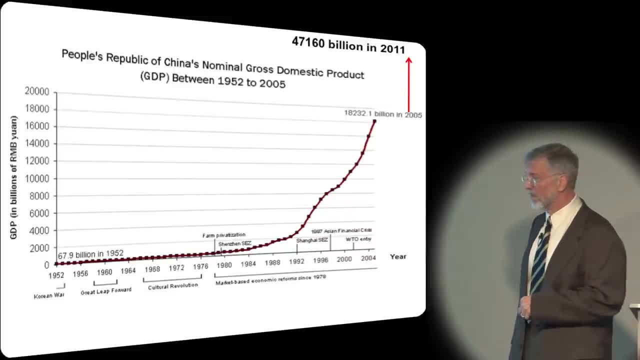 me into exile in Tibet for nine years. I said: wow, that's a really good excuse. Then he looked at me and said: what's your excuse? You know, it's like the 70s. I lived them. I don't remember them, But that was 1985.. And the Chinese? 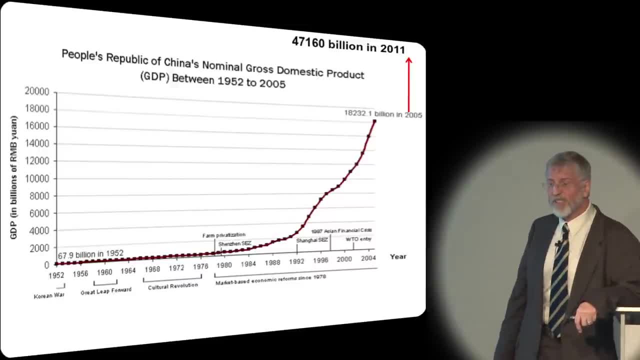 which you know this is like a quarter to a third of the world's population. they did us this huge favor during most of my lifetime. You know this is a hugely populous, hugely talented, hugely smart, ambitious group of people who decided to make themselves just. 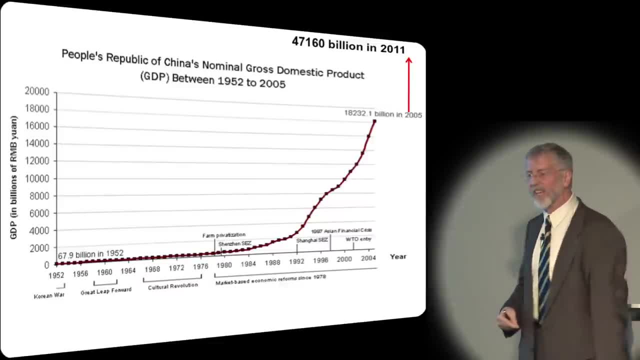 dirt, grumpy, Grinding poor for decade after decade after decade, And they didn't compete with us for resources or anything. They just wanted to be poor because you know that was their policy. And so this is the GDP of the People's Republic. And then about, unfortunately, Mao. 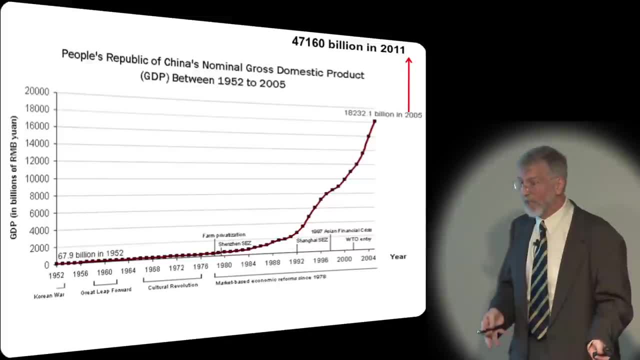 Zedong died. Mao Zedong, was this huge favor for us, believe me, in terms of carbon dioxide. They decided: oh well, let's do this. You're rich, We're poor, We're rich, You're rich, you're poor. 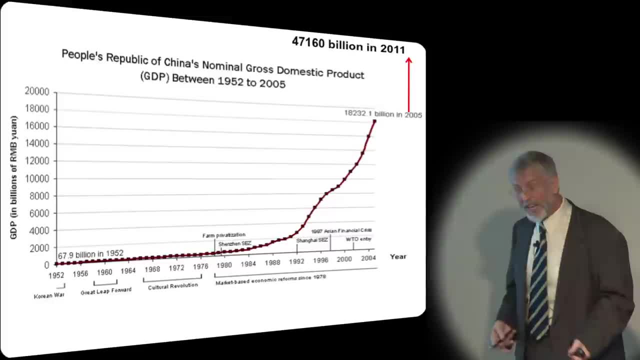 If we can't do this, oh well, why should we be poor anymore? Let's go make stuff and sell it and become rich And boom. This one only goes to 2004.. The actual GDP is 47,160 billion yuan. 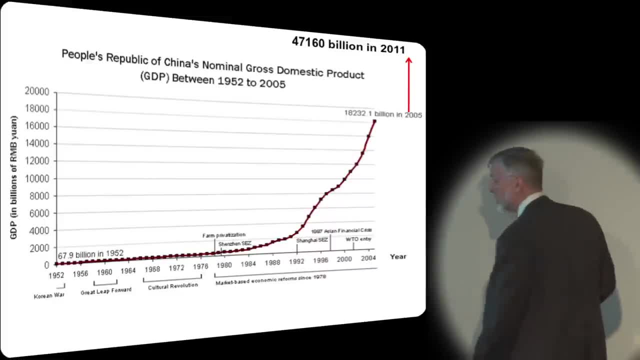 You know it's like above the second floor now on this plot And all these guys want the same sort of thing we want. You know, they want to live a middle-class lifestyle, They're going to live more rich, They want to drive a car, they want to have freeways and they want to have power. that. 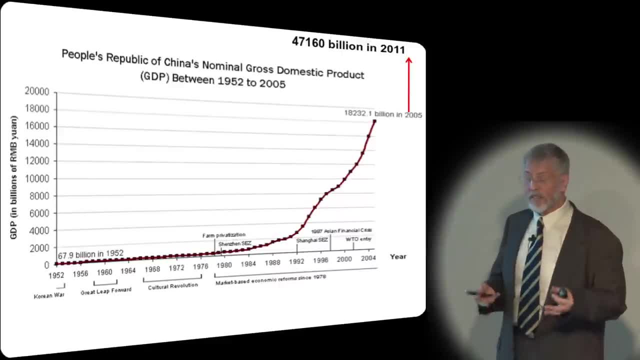 works 24 hours a day so they can run their air conditioning- because, believe me, it's just as miserable in Shanghai as it is in Pensacola during the summer. because you guys are at the same latitude, And so they're going to want to. they're producing a gigawatt-sized coal-fired power plant every. 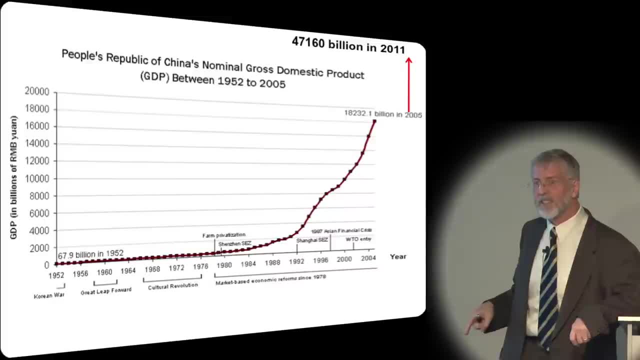 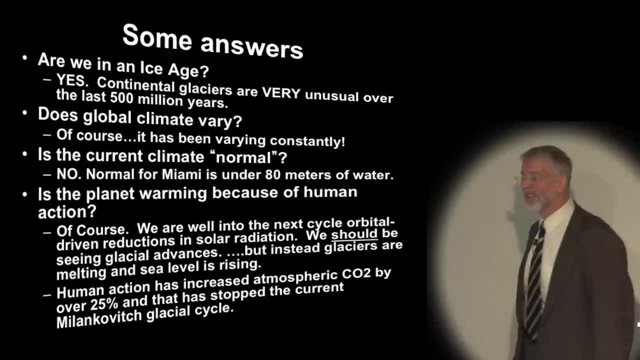 two weeks in China. So what do you think that's going to do to the carbon input? Okay, so some answers. Yes, we're in an ice age. If you look back over the last half-billion years, continental glaciation is very unusual. 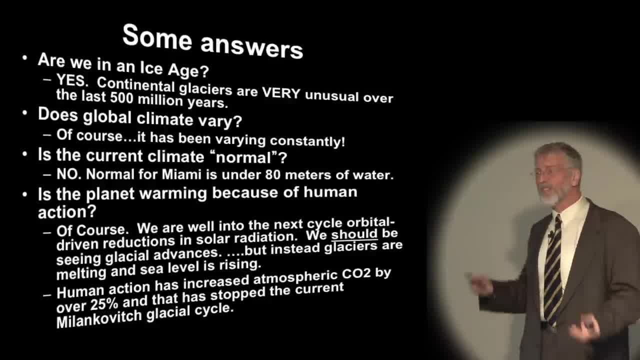 Very unusual. Does the climate vary? Of course it varies. It varies constantly. Is the current climate normal? No, normal for Miami is to be under 80 meters of water. Normal is not to have a Florida. Is the planet warming because of human action? 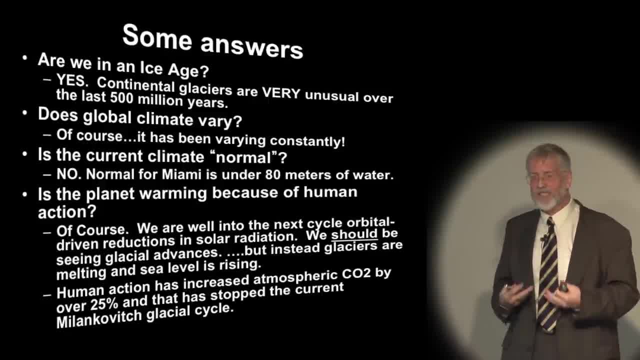 As a scientist, I am just floored that this is a political thing for political discussion. Of course it's warming. We are well into the next Milankovitch cycle. We should be getting advances in glaciation and we're not because we've been smart enough. 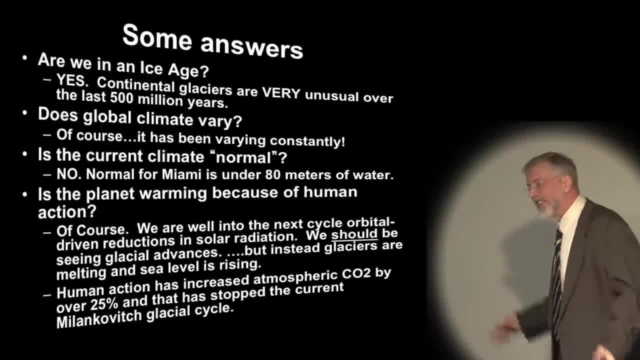 to. This is what we call geoengineering. We've been smart enough to change the atmospheric chemistry and redistribute the heat into the high northern latitudes and make up for this solar insulation that we're not getting. Human action over my lifetime has increased atmospheric CO2 by 25% and stopped the Milankovitch. 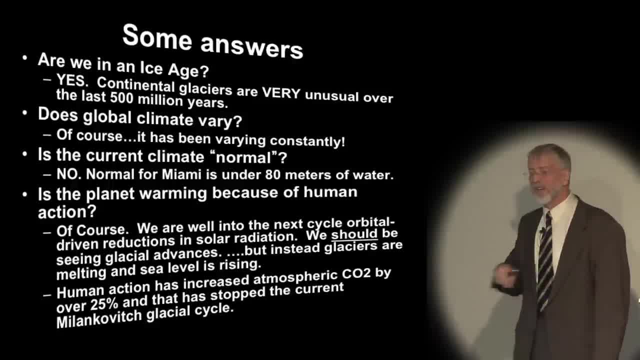 cycle in its tracks, but we have to recognize what we're doing. The downside of this is that if you look at Earth history And you have high levels of CO2, high levels of greenhouse gases, you don't have continental glaciation. 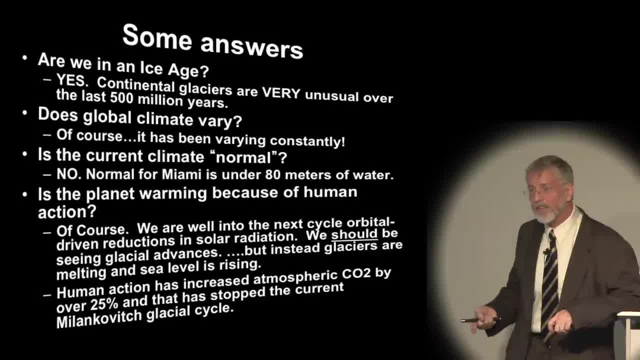 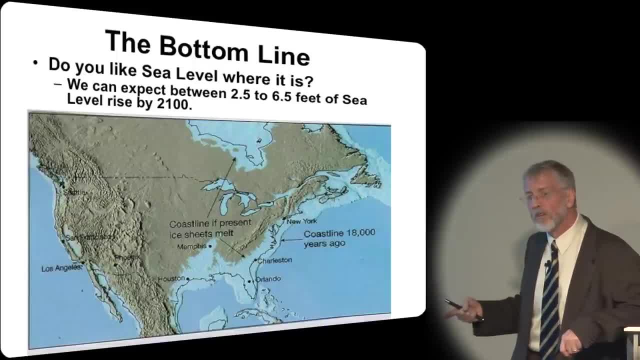 If you don't have continental glaciation, you don't have Miami. So the bottom line here is: do you like sea level where it is Yes or no? If you don't care, then we're done talking. Go and drive your Hummer. 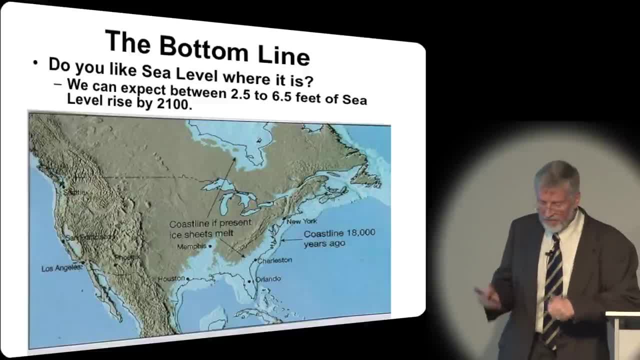 Now, as I tell my class, this is not my problem. I'm going to be dead before the sun. Remember, this is going to be a serious problem. This is my children's problem and their children's problem. You can expect sea level rise of between about 2.5 to 6.5 feet by 2000,. over the next 90 years. 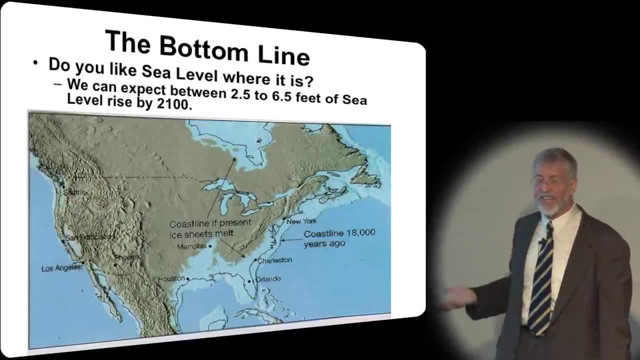 Most of that is going to be non-linear, so most of it's going to occur toward the end of the century. The unknown here is the dynamics of- I'm sorry, The dynamics of glacial collapse Now, luckily in Greenland. Greenland is kind of bowl shaped so most of the glaciers are. 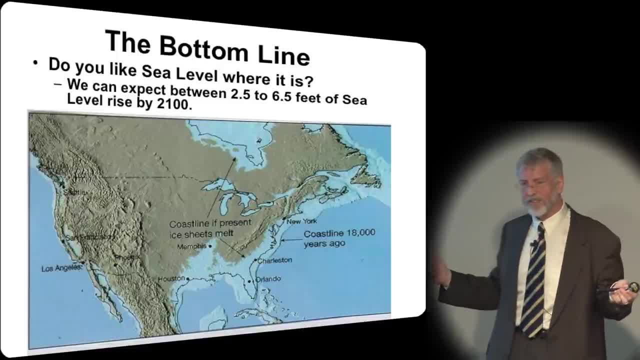 surrounded by mountains and there are only a few exits, And so it probably won't collapse really catastrophically. You can see things in the geologic past where you have catastrophic glacial collapse. The Laurentide Ice Sheet in Canada Catastrophically collapsed and melted. 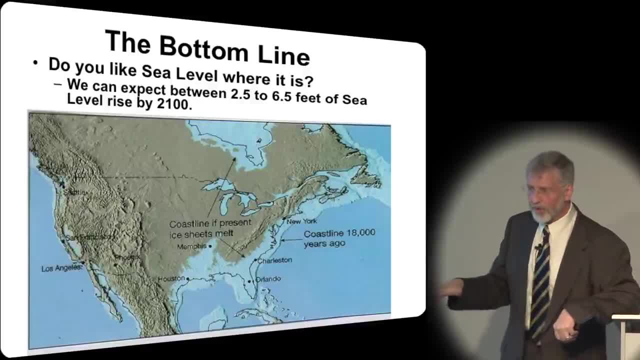 If any of you have ever been to Quebec or Montreal, you can see the St Lawrence Valley. If you look at the St Lawrence Valley, the St Lawrence occupies this little tiny strip on this big, huge, flat plain of a valley and you can see mountains off in the distance. 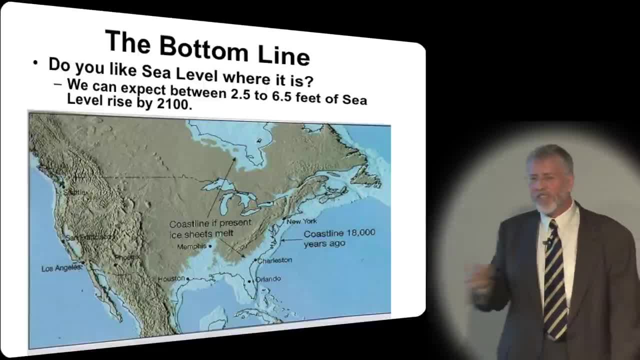 one way and mountains off in the distance the other. That whole thing used to be a solid river when the Laurentide Ice Sheet collapsed And what happened was over a thousand years You increased sea level by 30 meters, So you can get really rapid sea level increase. 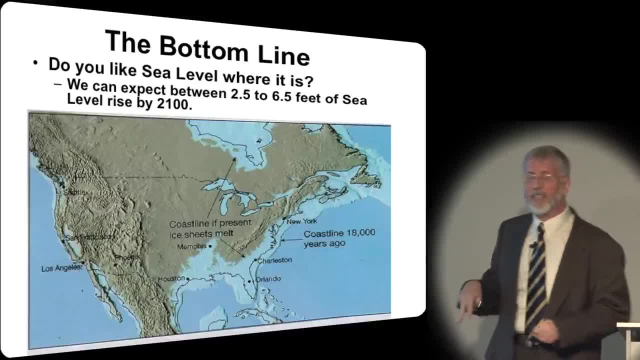 So do you like sea level? Because what's happened is that we've already gotten to a level where the Greenland Ice Sheet is in disequilibrium with the CO2 level in the atmosphere. It's going to melt. The question is how fast. 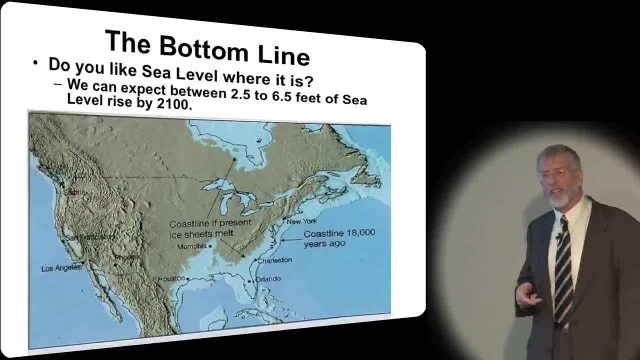 And we're working on that. We don't know quite yet, But this is going to be a problem for future generations. My students then say, oh, thanks a lot. I say, well, hey, you know, I'm just passing it along. 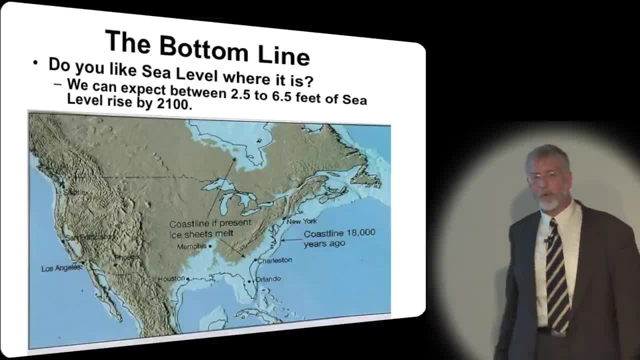 My father left me the Cold War. His father left him World War II. That's what generations do. They didn't appreciate that. but what the hell? So anyway, just to give you a little bit of perspective. I don't know. 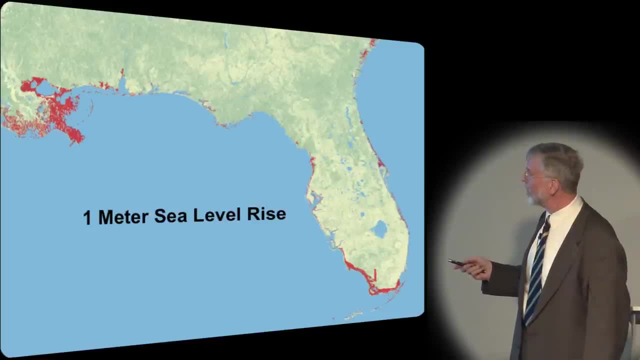 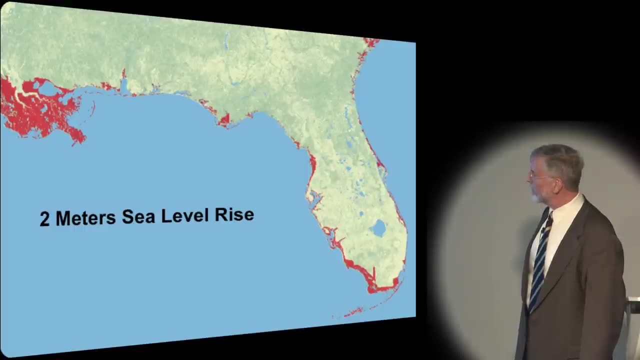 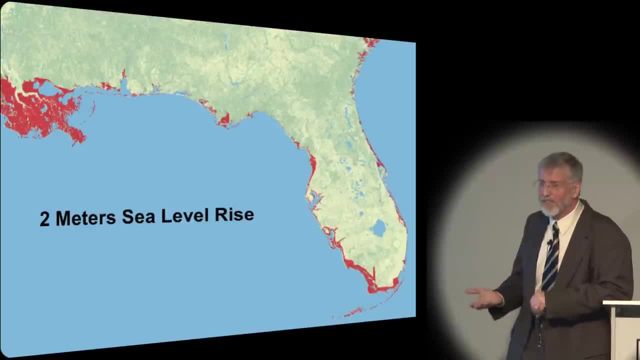 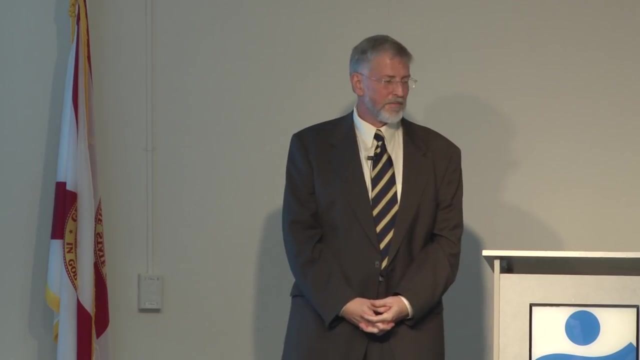 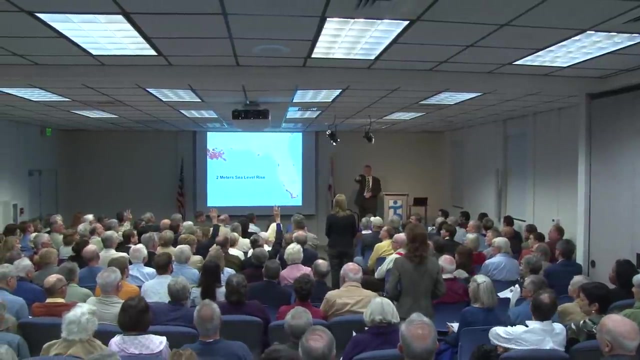 Ask yourself what percentage of the assessed valuation of Florida is within 10 feet of sea level. So, anyway, I will leave you with this happy thought. I'm going to stop here. Thank you very much, And I will take questions. Yes, ma'am. 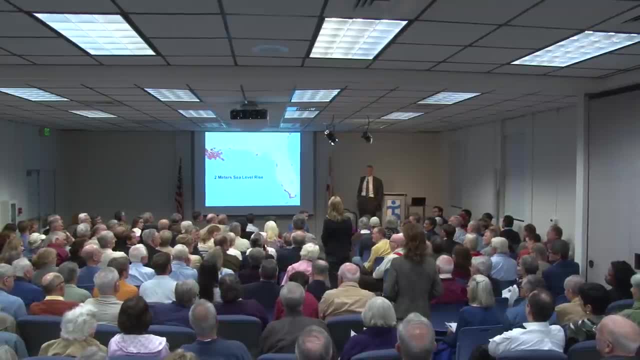 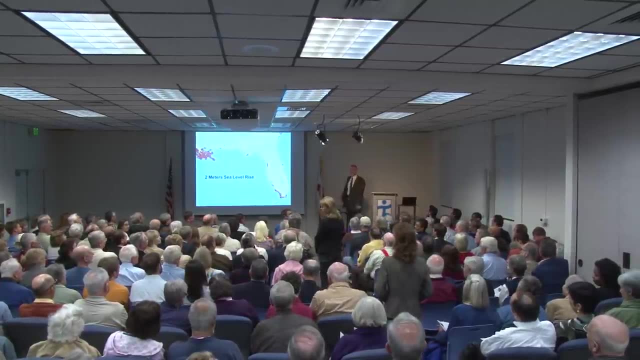 Thank you for putting the bell on the cat. I know other people have been doing it too. Well, the reality is a lot of fun sometimes And the canaries have been dying in the mines. Thanks, and I'm thinking of the Southern Hemisphere especially. 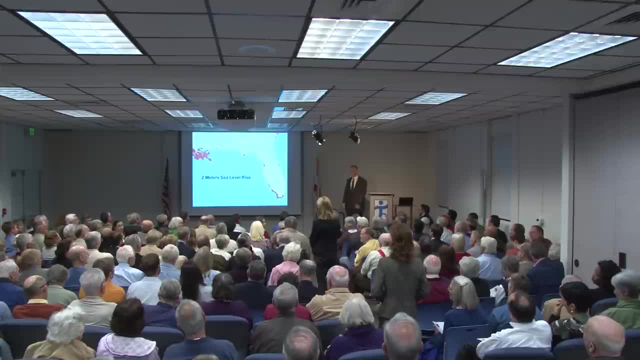 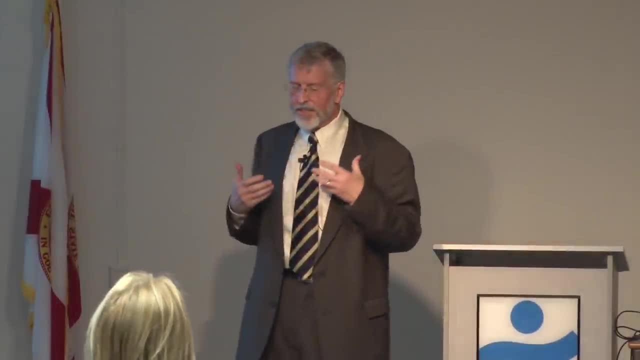 the droughts, the dying of cattle, the dying of people. are they not feeling it before we are? Well, the problem is, I look at this as a geologist, And so the I hate to sound unsympathetic. but the average age of a species is about three million years in geologic times. So you get extinctions all the time And you can argue till you're blue in the face if this extinction or that drought is caused by global warming, because that's a modeling problem. 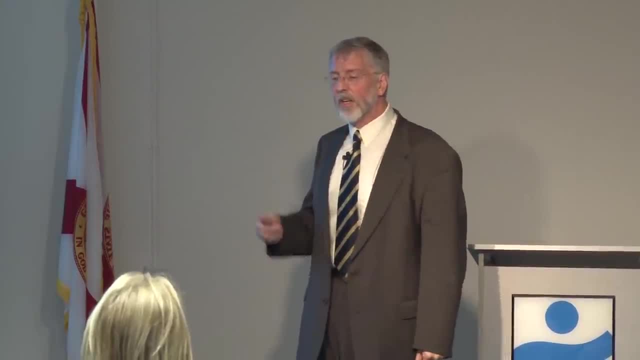 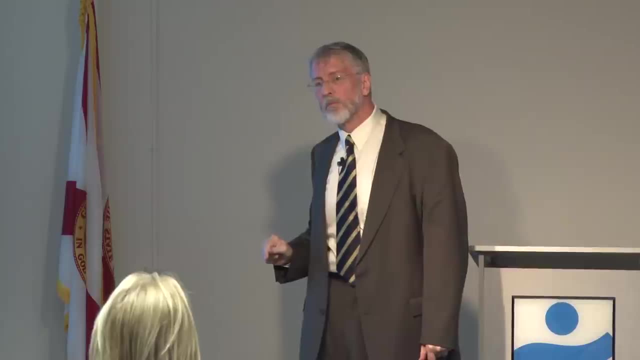 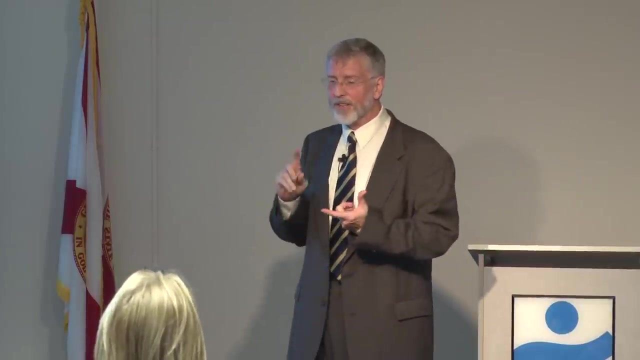 and it doesn't have a definite answer. If you look in the geologic record, what you can read out is that sea level is correlated with CO2. And so this is what I can definitely point to as solid evidence. Yeah, I agree with you that droughts 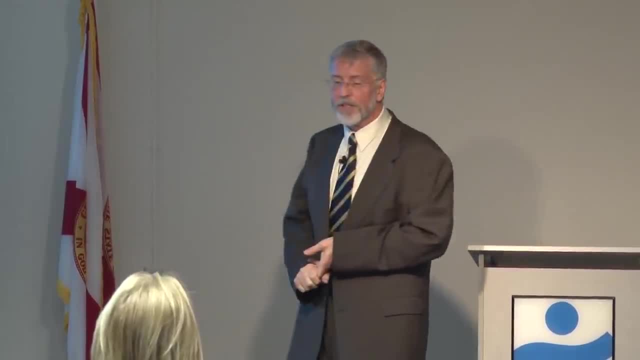 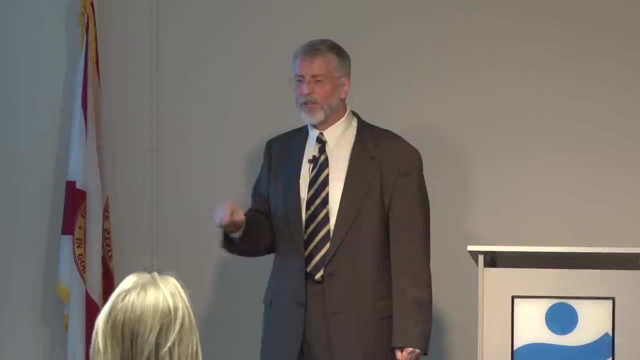 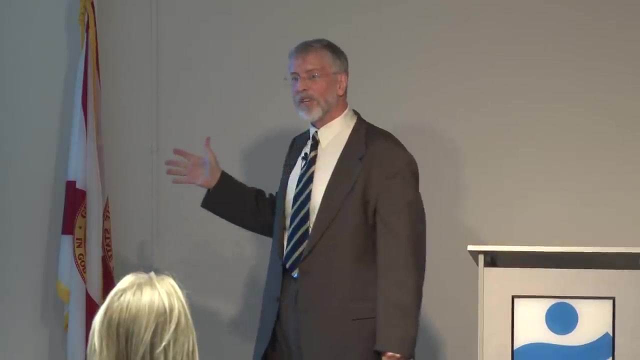 changing climate conditions, more rapid extinctions are all part of the equation. But you can't really point. it's sort of like smoking and lung cancer. You can't say, well, that's the smoking gun right there. This is the smoking gun that I know about. 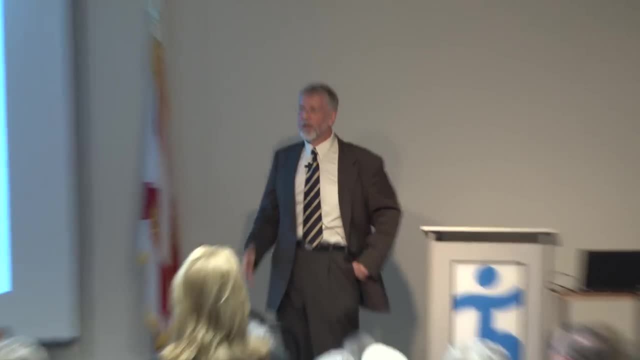 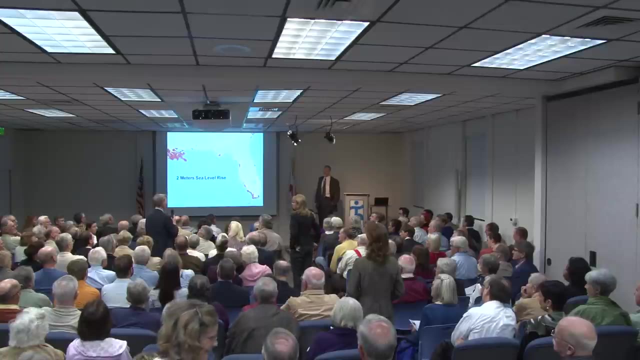 And also I'm a rock guy, so this is what I know about. More questions Over here. Thank you very much for an engaging lecture. Sure Petzgal was blessed A month ago with a speaker named John L Casey. 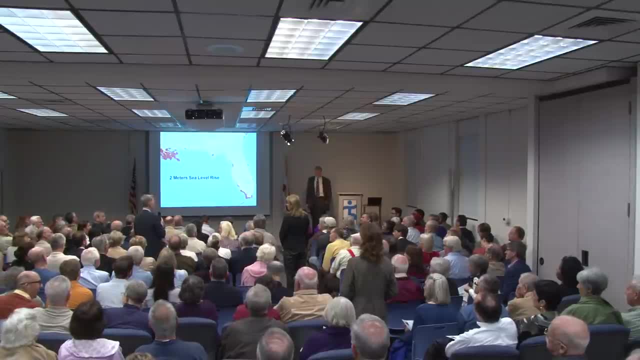 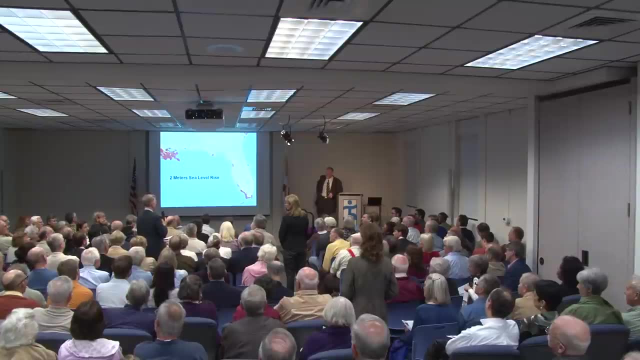 who's written a book called Cold Sun And his premise is that there's a 206 year cycle And, like you mentioned, there's a we're in the phrasing end of it And he says there's actually some kind of a sun hibernation going forward. 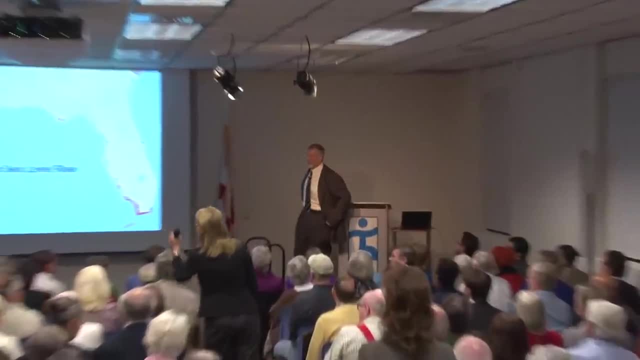 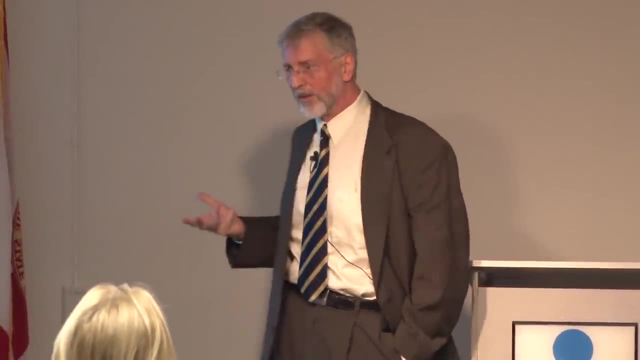 Do you know anything about any sun hibernation? Yeah, there's a. you get a variation in the sunspot cycle And there was a period called the Maunder Minimum where basically you had no sunspots, And so that makes things a little bit more complicated. 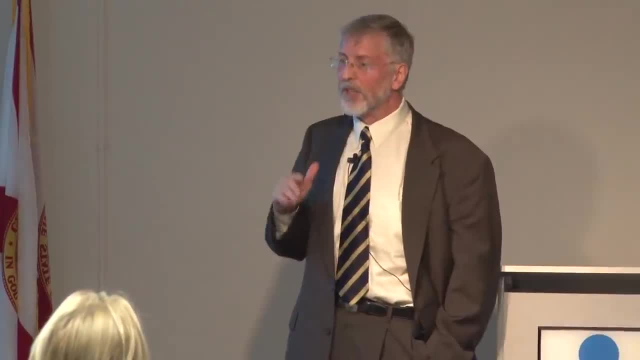 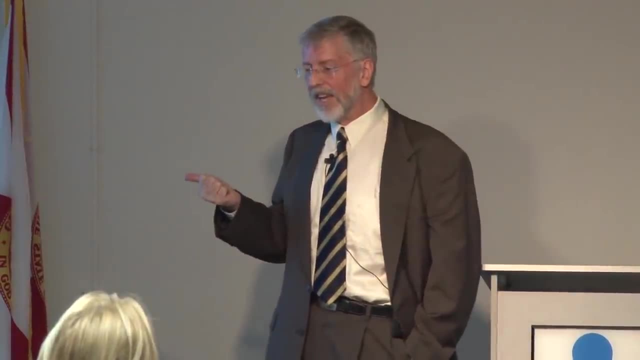 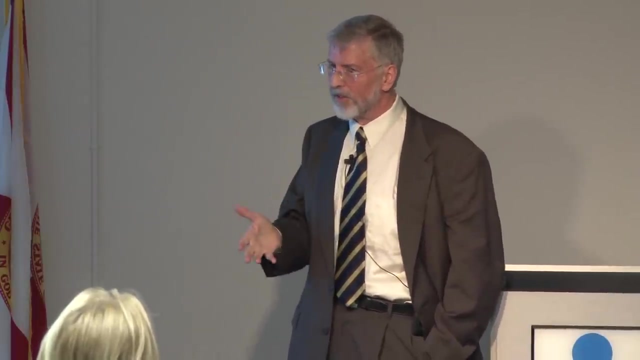 It's a little bit colder. That doesn't make things anywhere near cold enough to do the to affect these glacial cycles. As I said, that sort of thing is in the noise, Whether there's actually this 200 odd year solar cycle. 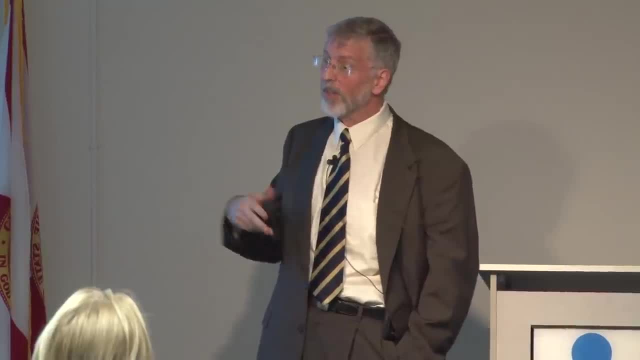 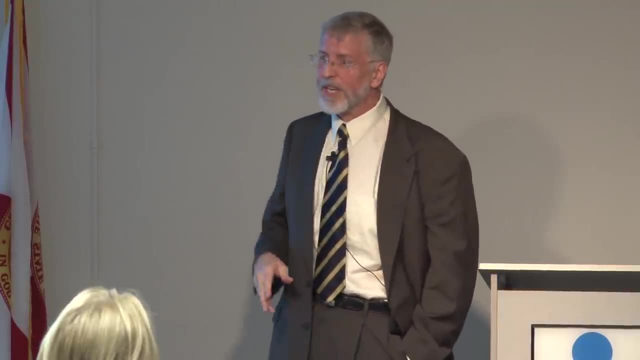 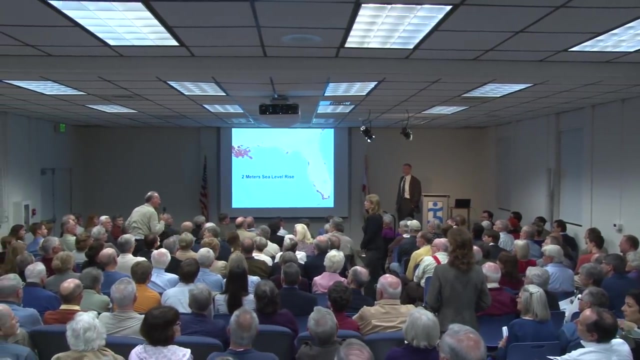 is pretty speculative stuff And I've seen evidence for and I've seen pretty strong evidence against, so It might be, but it's in the noise. Yes, sir, Let me ask you to combine two areas of your expertise. Okay, 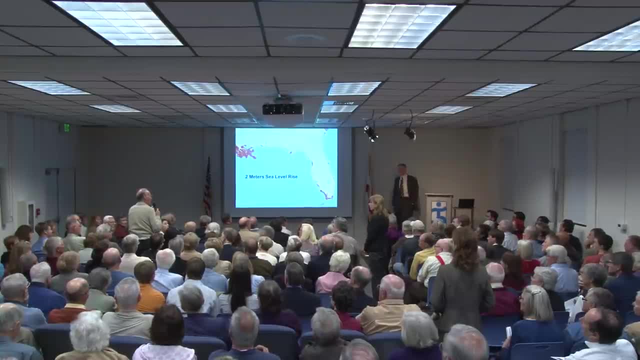 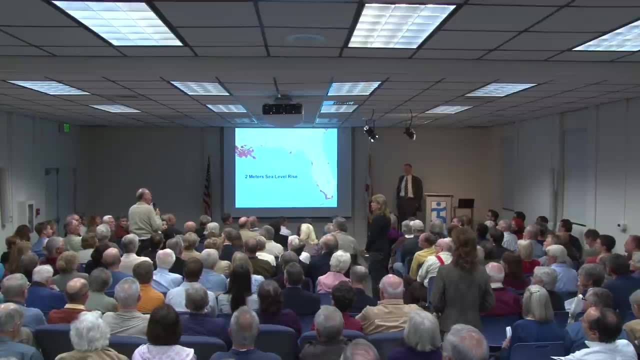 I have been reading that the polar glaciers on Mars are actually shrinking And I don't know if that's true or not, but can you use Mars as a model? you know, absent all the anthropogenic effects and just look at some of the the major effects. solar irradiance and the global mechanics and so forth, and I don't know what you'd have to do. maybe have boreholes on Mars or something to well, you know, that's not beyond. well, actually, there's a quick answer for that. Mars is actually more variable in its insulation properties than the earth is, and so 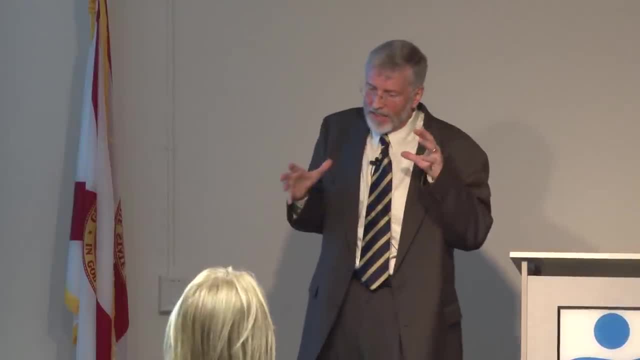 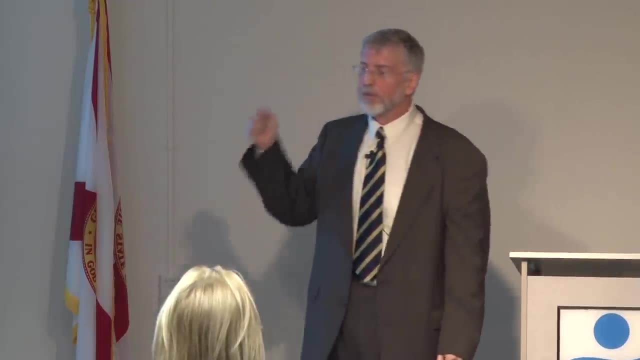 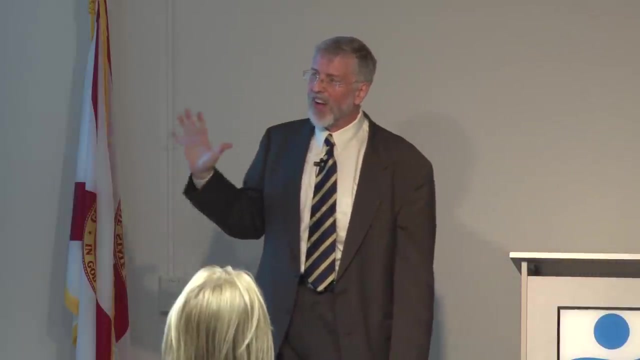 people have done this work and Mars varies so much that that you you actually can change the tilt to about 45 or 50 degrees and with that happens the polar caps melt, put all that put lots of carbon in the atmosphere and you increase atmospheric pressure by a factor of five. so people have thought 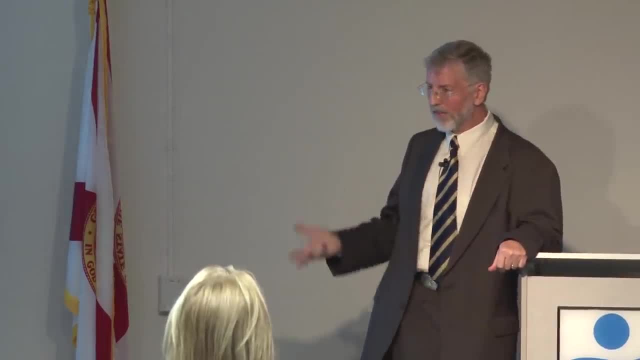 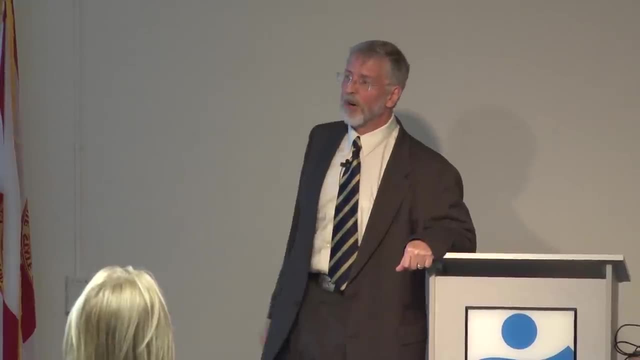 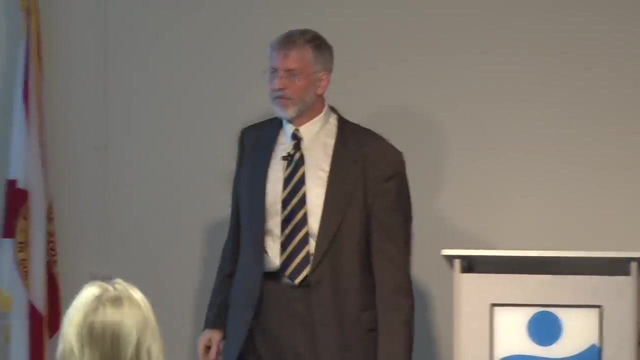 that during those periods, you might have enough atmospheric pressure to have, like you know, bacteria and critters and things, and that's one thing that NASA is looking for. so, yeah, we've applied this to Mars and that it does work, and Mars is actually kind of in the depths of its ice age right now. yeah, well, wait for. 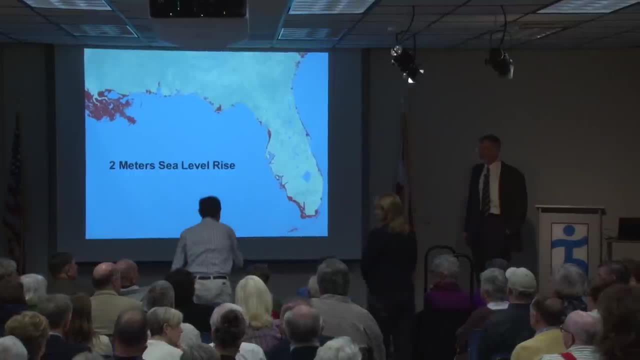 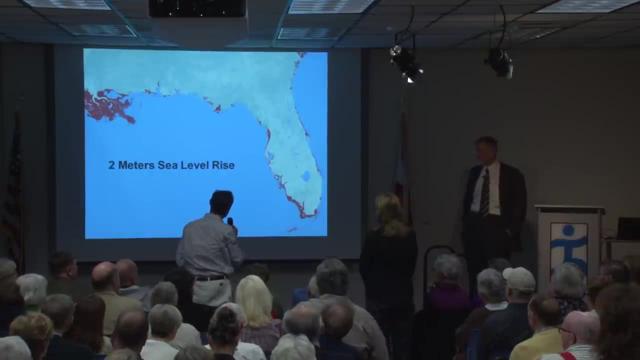 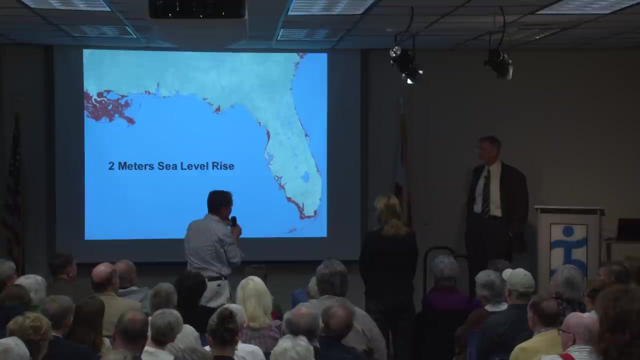 it for the wait for the microphone. loved your speech, thank you. thank you got a lot out of it, but I need to think this through. we can say this, but there is no proof that that's going to happen. we can, we can go through the math. we can do all. 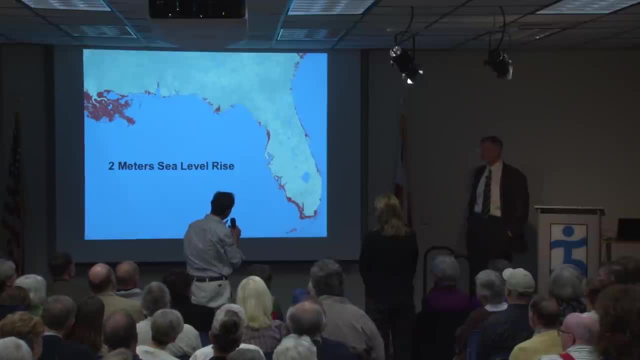 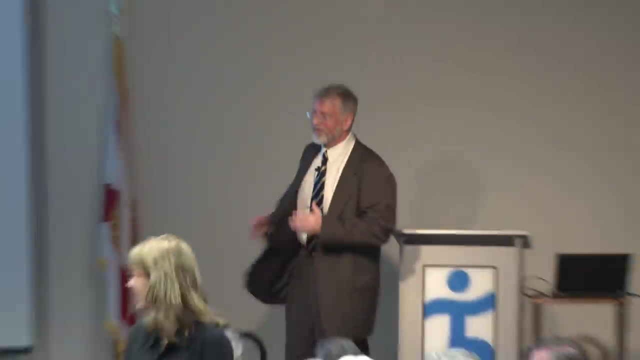 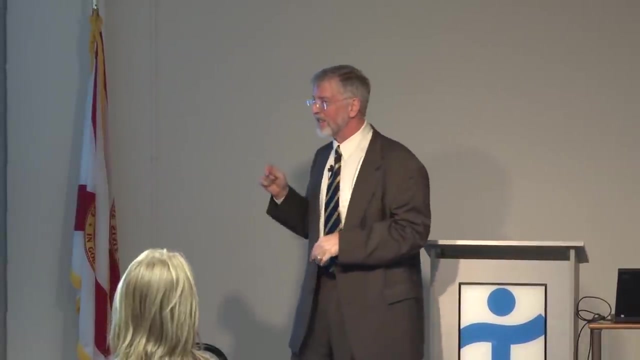 the scientific evidence. we can but show me the numbers. you showed numbers and I appreciate that I can make pretty graphs. I don't think that's gonna happen. okay, it's, that's fine with me. see, I don't do any mathematical modeling. what I do is I look at past epics and Earth. 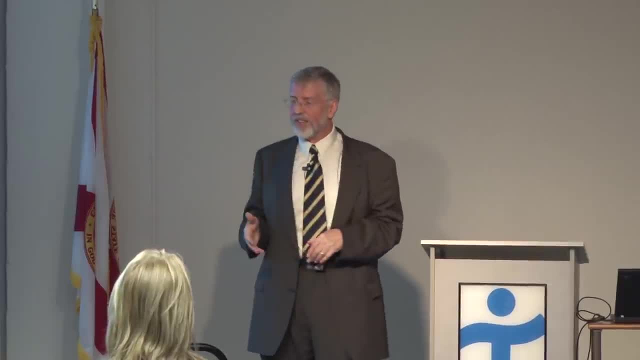 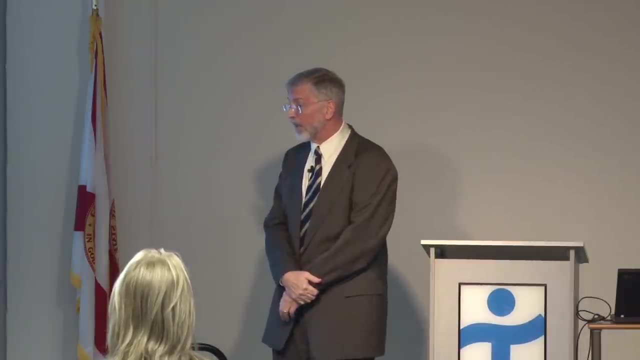 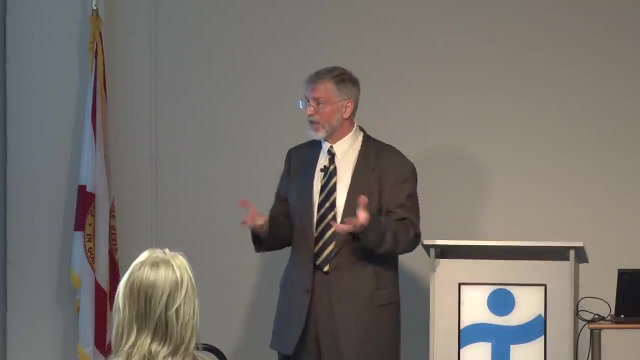 history where you've had elevated co2. when you have elevated co2, you have higher, higher sea levels. and you can, you can, You can do the Milankovitch modeling fairly easily, and there's a number of sites that do that for you. So take a look at it yourself. 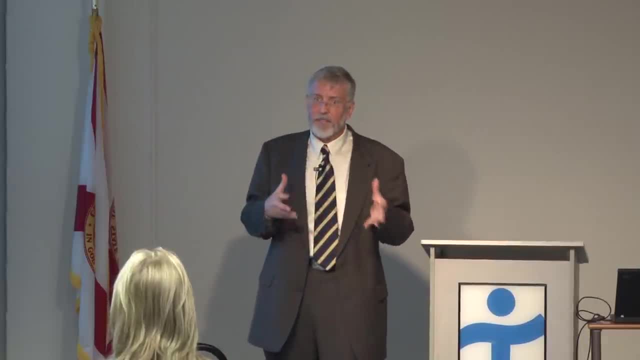 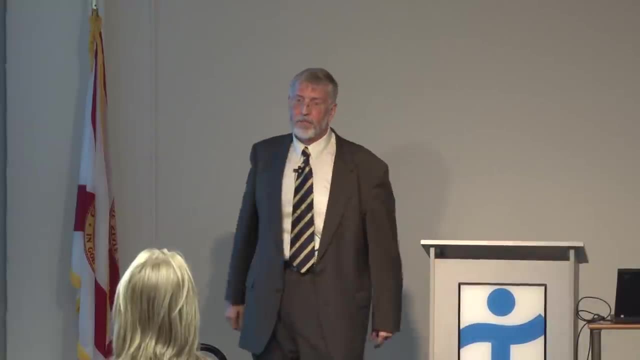 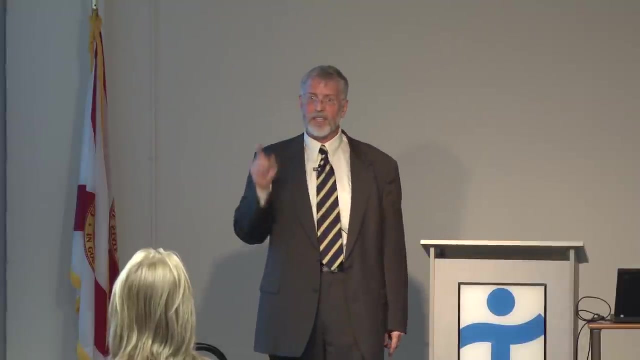 As I say in these past, climate epics. don't believe me, you can go and look at these things yourself. One of the things about scientists is we don't believe in theories. We observe them, And so we're always constantly testing them.